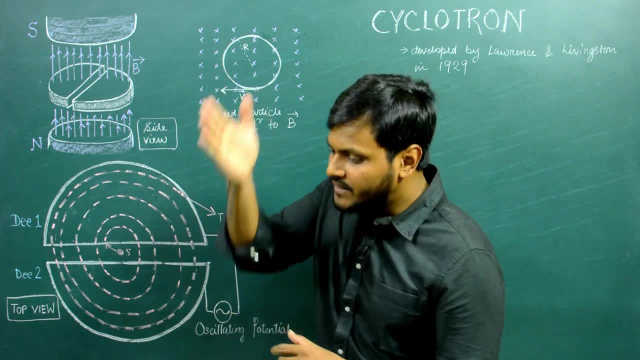 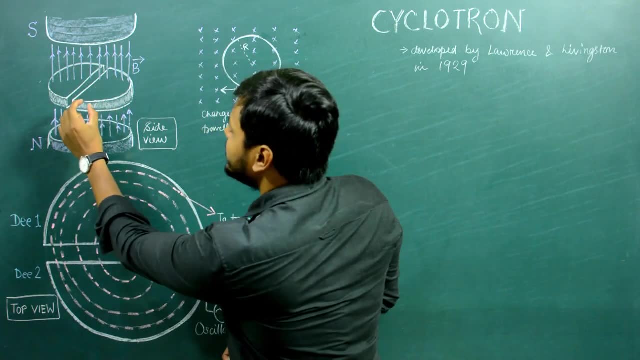 which if, let's suppose, I take a cylinder and cut it along its diameter. So if you have a cylinder and you cut it along its diameter, you basically separate the cylinder into two halves, creating a space along its diameter. So you basically have the semi-cylinder. 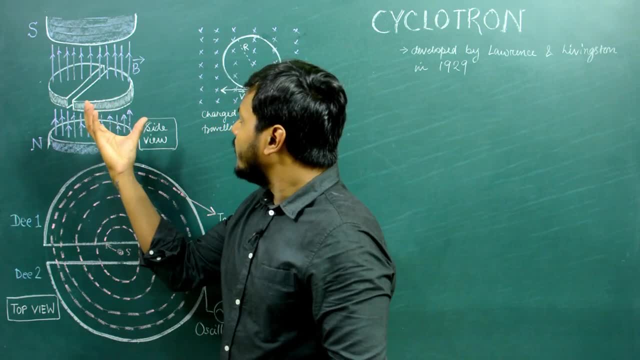 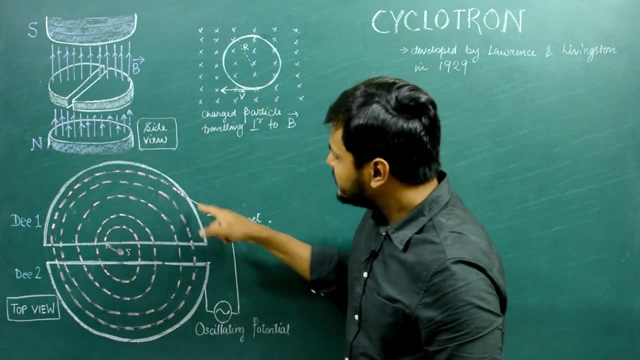 and the semi-cylinder, which is basically separated by a small space. thus they are not touching each other. So here you have one half of the cylinder which is known as D1, and the other half of the cylinder, which is known as D2.. They are separated by a little. 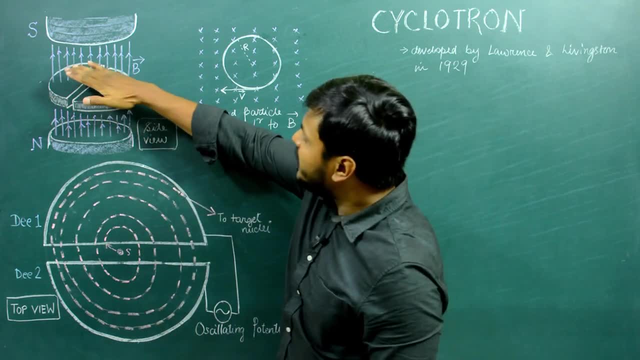 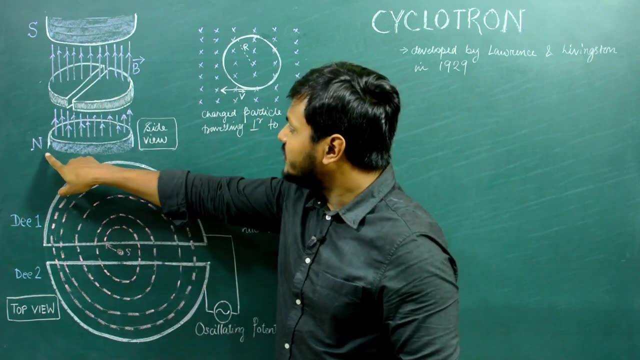 bit of space, and this entire setup is placed perpendicular to magnetic field lines, which are generated by some sort of an electromagnet, where N here is the North Pole shape and S is the South Pole shape. That's how, If the networks are able to interact, They do this undefined. 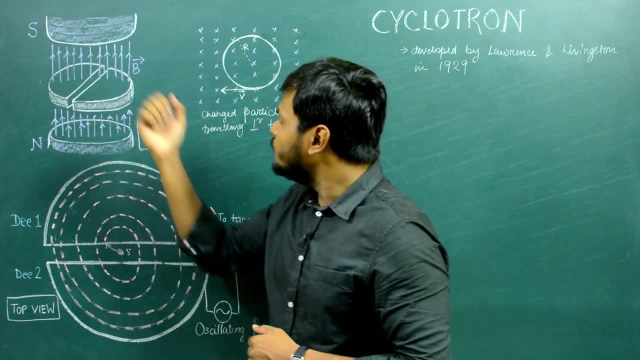 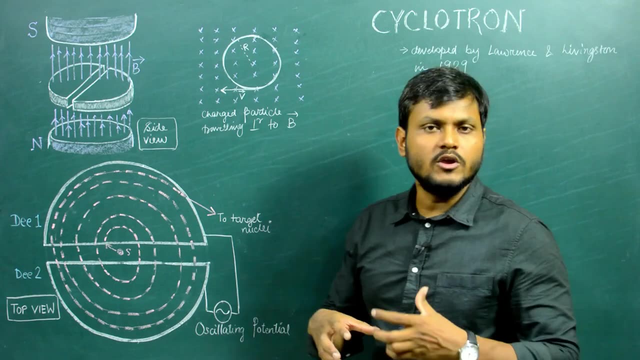 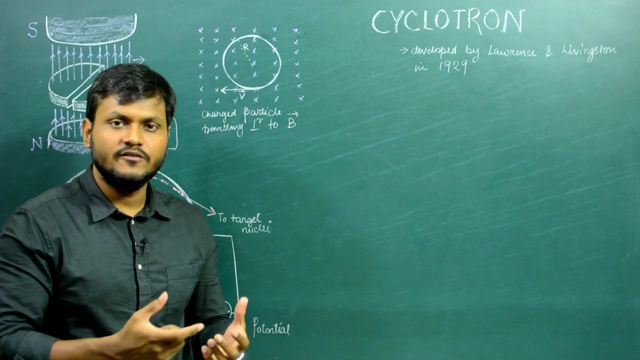 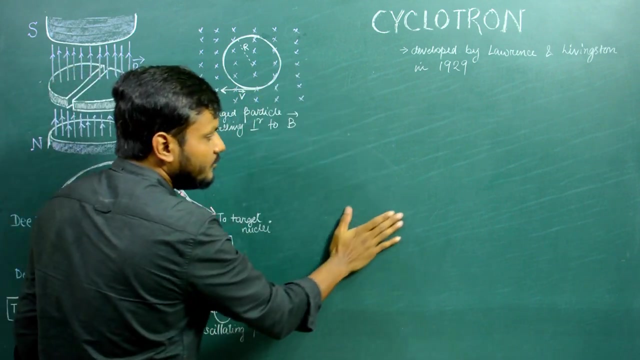 the south pole. The purpose of the magnetic field line is to make sure that the charged particles inside the cylinder traverse a circular trajectory. Now you must know from your concepts of electrodynamics that whenever a charged particle is traveling perpendicular to a magnetic field, then it usually traverses a circular trajectory. So, for example, if you have this plane of the 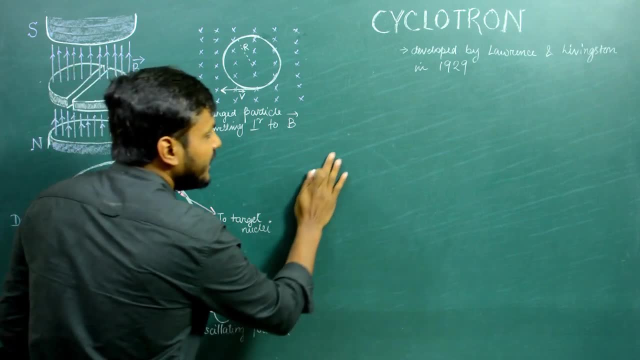 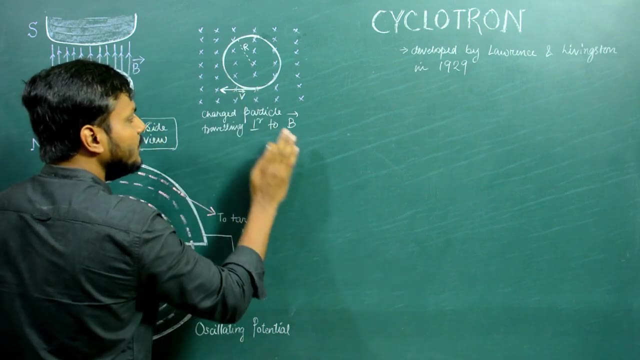 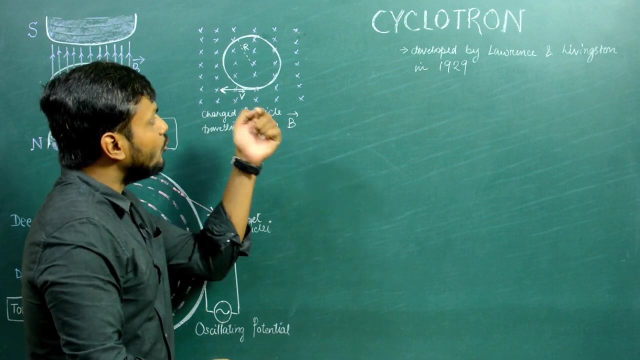 blackboard that I basically have and in this plane a charged particle is traveling with a velocity vector of V. If a charged particle is traveling on the plane of this blackboard with a velocity vector V and let's suppose magnetic field lines are protruding out of this board perpendicular to the plane of the board, 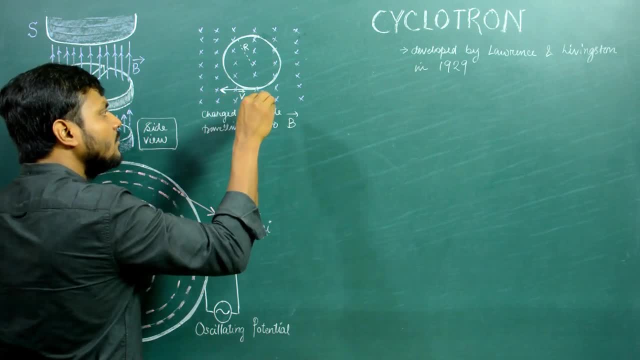 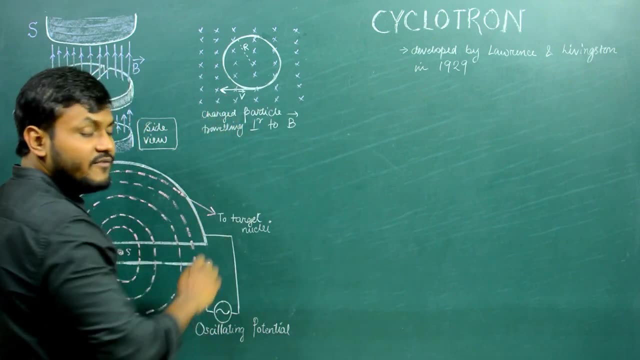 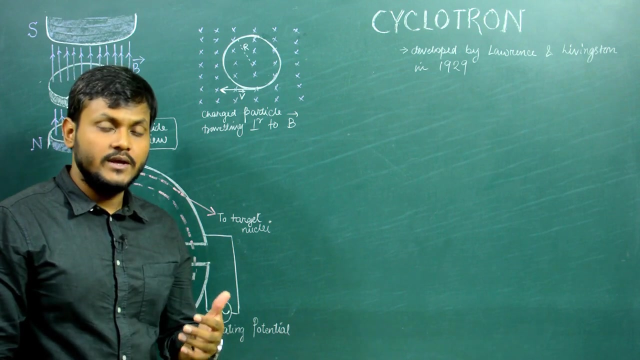 Following magnetic field lines are protruding out of this board perpendicular to the plane of the board. in that case, the magnetic field line B will be perpendicular to the velocity vector V. In such a case, the trajectory of the charged particle comes out to be a circular trajectory. Now, if you do not know why this is so, then I: 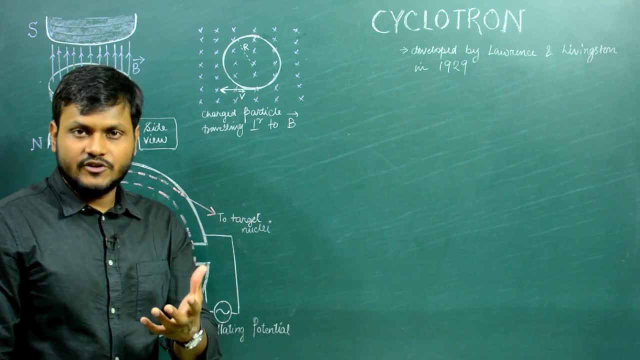 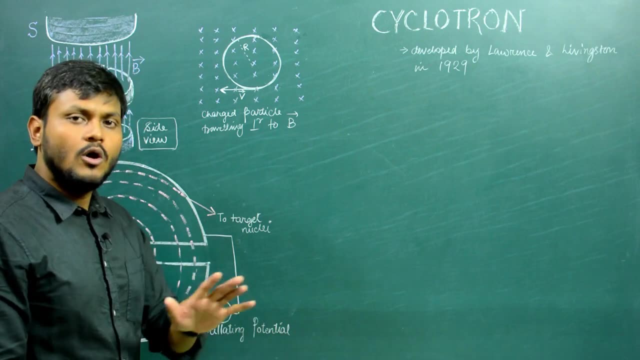 have created another video where I have discussed the different kinds of trajectories created by charged particles in the presence of electric and magnetic fields. You might want to check that one out. But if you are confident with this idea that a circular trajectory is exhibited by a charged 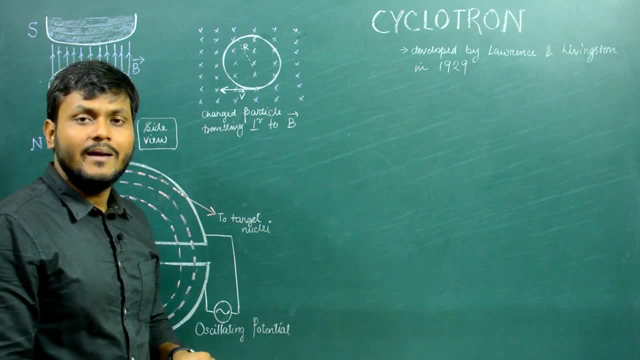 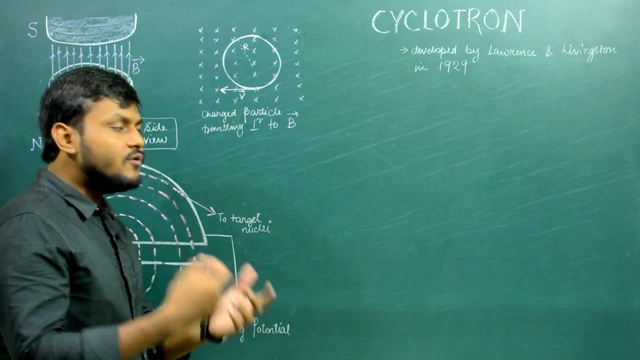 particle whenever the velocity vector is perpendicular to the magnetic field line, then we can move ahead. So basically, the force law which basically gives us the force experienced by a charged particle in the presence of a magnetic field is given by the Lorentz force law. 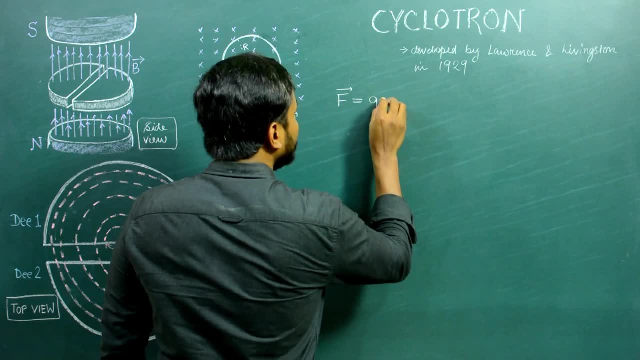 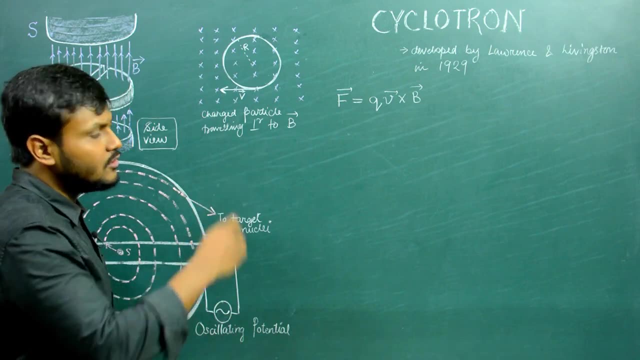 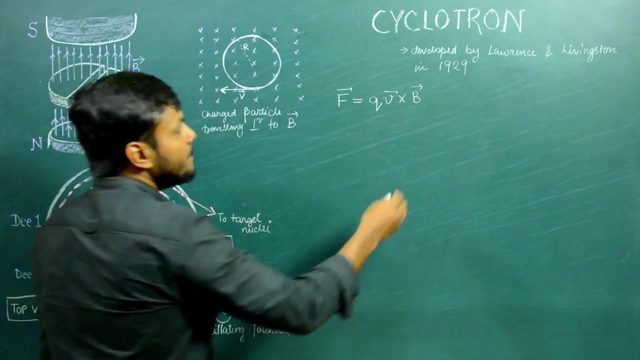 which says that the force experienced by a charged particle Q is basically equal to its velocity vector V, multiplied by the magnetic field line B. This is a cross product, But in this case the magnetic field line, the velocity vector, are perpendicular, So it is a 90 degree angle. So this can be written as QVB. 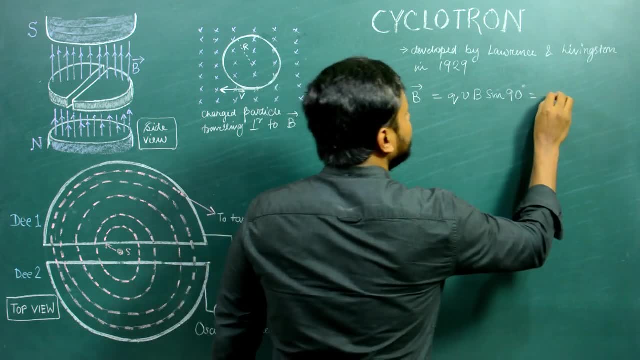 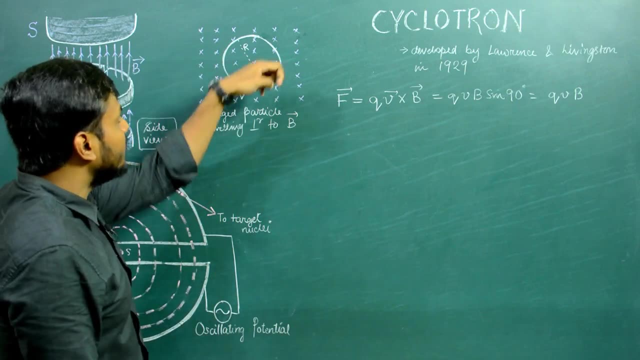 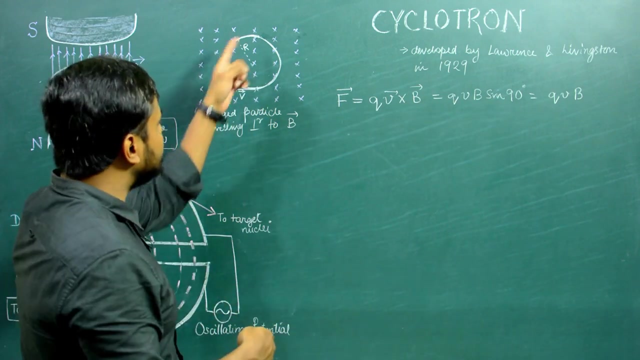 sine 90 degrees. So this can be simply written as QVB. Now, this is the force which creates this sort of a circular trajectory. So we can say that this force is basically responsible for the centripetal force which keeps the particle in a circular motion. So we can say that Q. 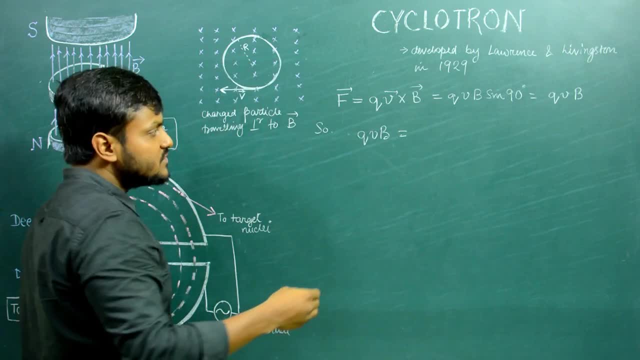 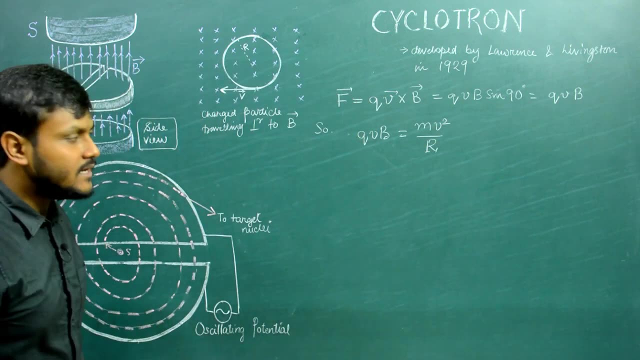 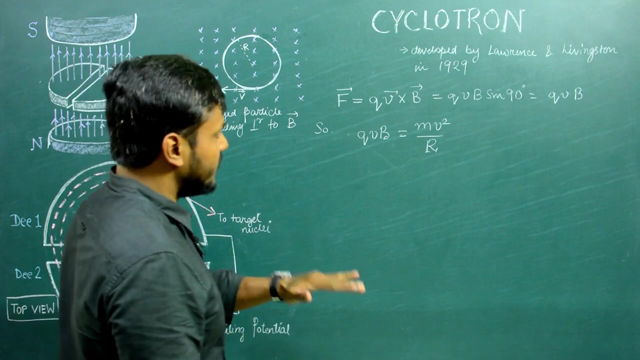 V, capital B, which is the Lorentz force, is basically responsible for the centripetal force, MV square upon R that keeps the particle in circular motion. From here we can calculate different sort of physical quantities associated with this kind of a motion. For example, I can: 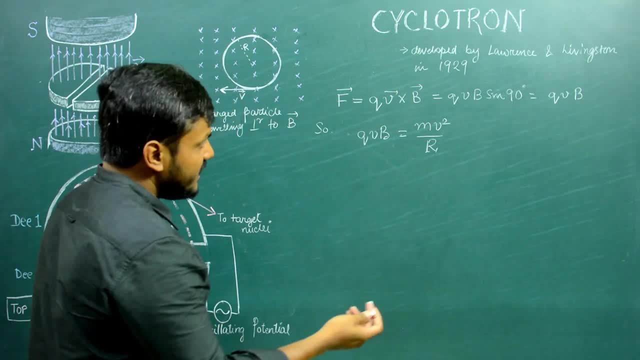 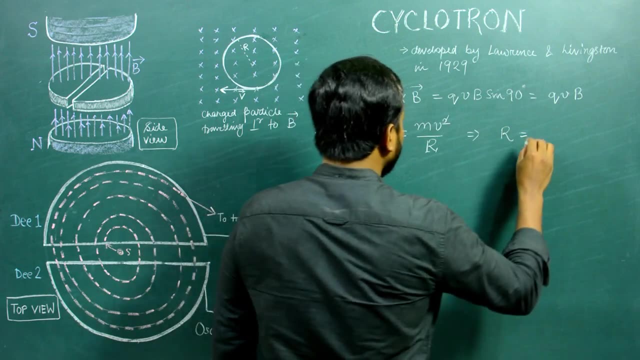 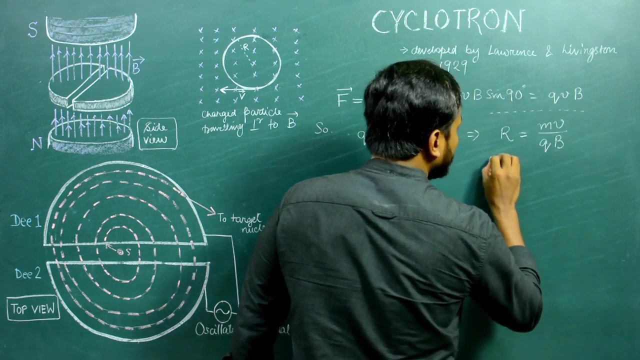 calculate the radius of this kind of a circular motion. So if V and V gets cancelled and I end up getting capital, R is equal to MV V divided by QB. So this is the radius of any charge particle having a velocity V and 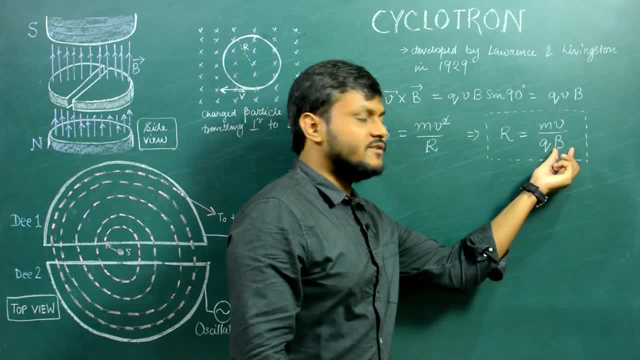 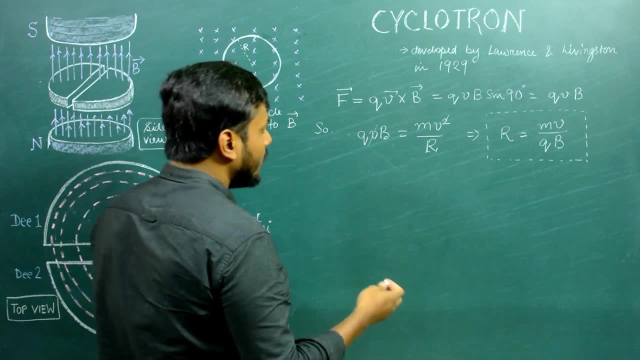 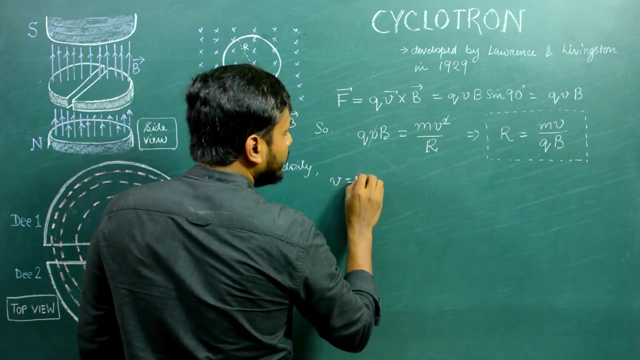 mass M and charge Q, but in the presence of a magnetic field B. So this is a radius of the circular trajectory. I can also write this equation to look at the velocity. So the velocity- the velocity is basically V- is equal to Q, capital, B, R. 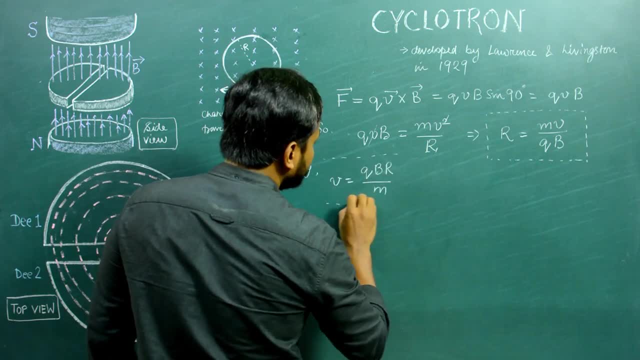 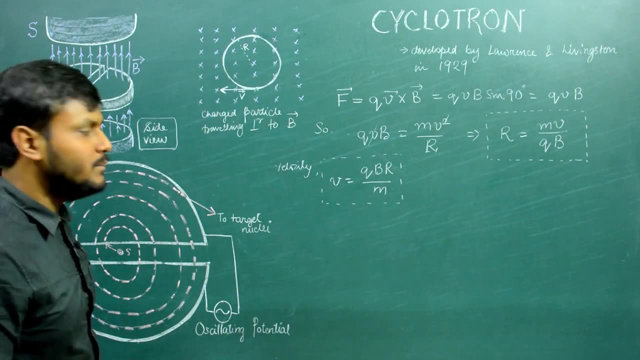 r upon m right. This is basically the velocity. So from velocity I can find out the total amount of time period it requires for the charged particle to make one complete revolution. So the total amount of time period to make one complete revolution is nothing but the circumference. 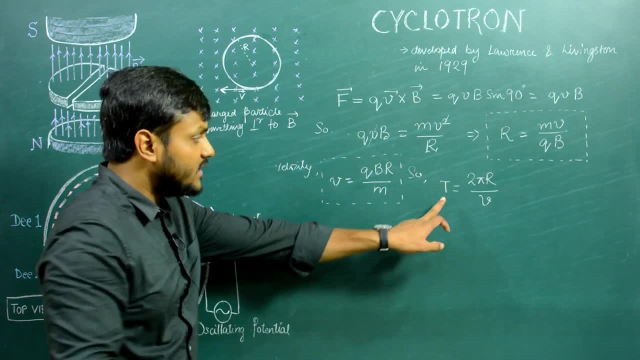 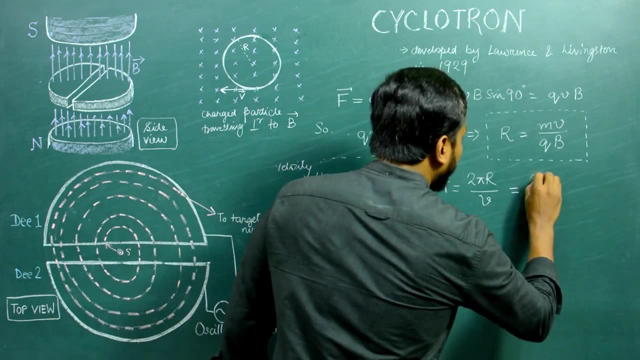 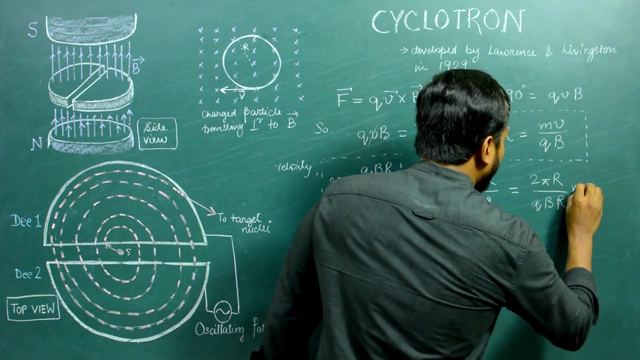 2 pi r divided by the velocity. yes, Time period for one complete revolution is the circumference divided by the velocity. So this is basically equal to 2 pi r divided by the velocity. We have just now obtained q capital B? r upon m? r? r gets cancelled, You basically end up getting 2 pi m. 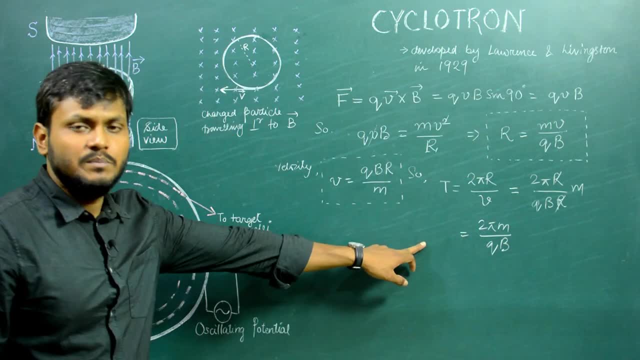 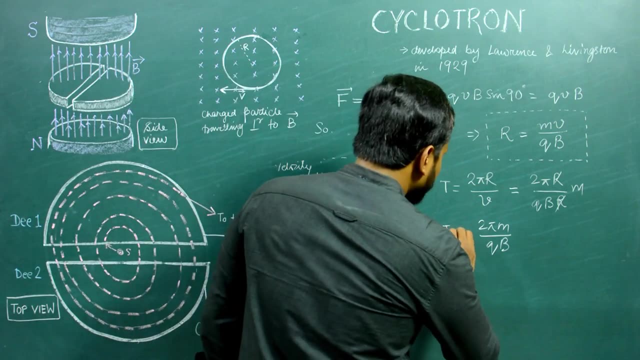 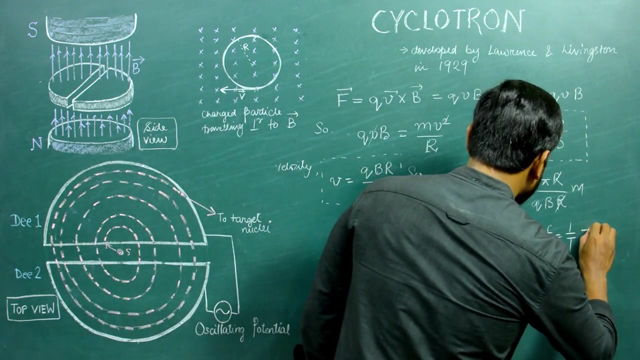 upon q B. So this is the time period. So if this is a time period, I can easily calculate the frequency of this kind of a revolution. So the frequency of revolution is nothing but f is equal to 1 upon capital T, which is nothing but the inverse of this, which is q B upon 2,. 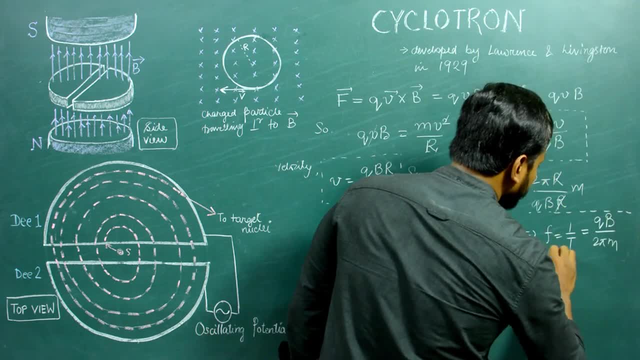 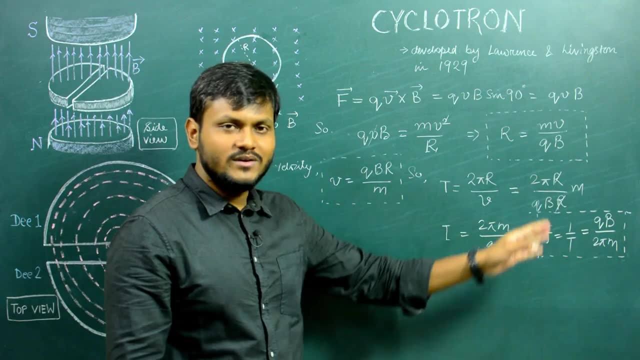 2 pi m. So this is the frequency of the revolution of this particle as it goes along in a circle. Now, why have I obtained these physical quantities? Because, as you will see, it will help us gain a little bit more perspective in understanding what is happening in the 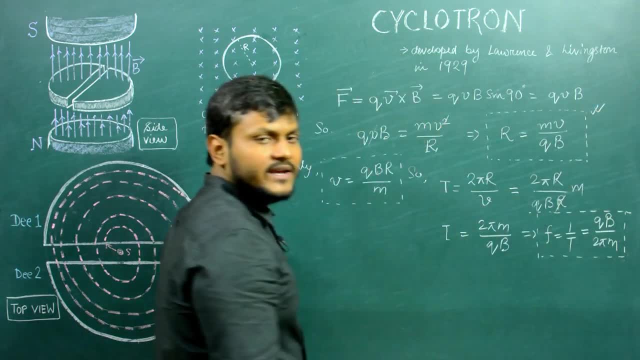 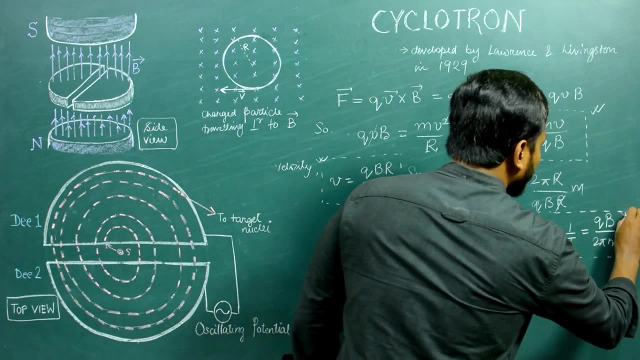 cyclotron. So this is the radius when it's a charged particle executes a circular trajectory. This is the velocity for the charged particle to have this sort of a radius And this is the frequency with which a charged particle executes a revolution per unit. 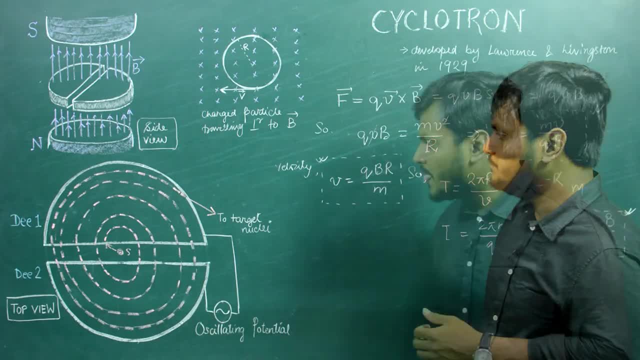 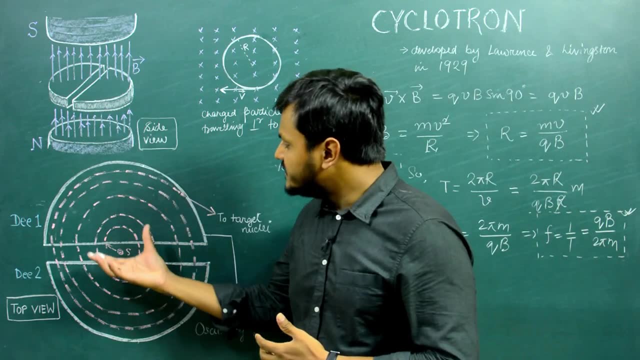 Now let's come back to the cyclotron here. So how does the cyclotron accelerate the charged particle to such high velocities in the first place? So here you have the cylinder, which is separated in the middle And the half. both these two halves are connected to the opposite polarities. 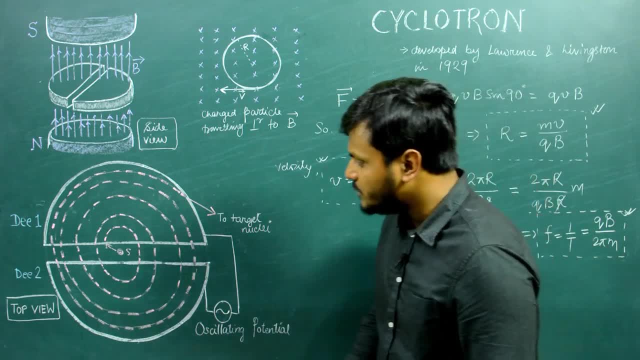 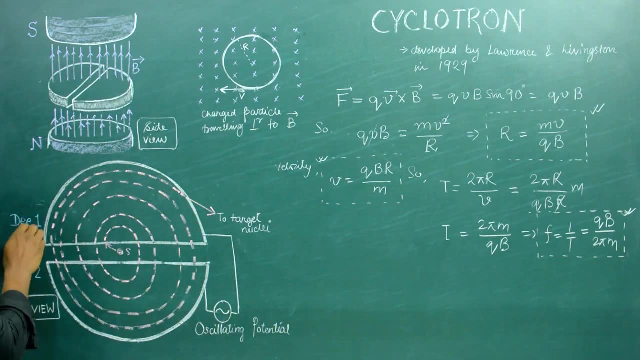 of an oscillating potential. Why an oscillating potential? Because if let's suppose at any given instant in time the first half, the d1, is at a positive potential, In that case the second half will be at a negative potential And therefore there is going to be an electric. 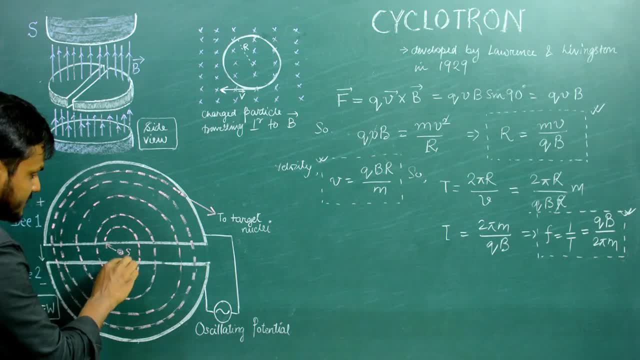 field line between these two d's in this space here, After some period of time, when the polarity of the oscillating potential reverses, this is going to become negative and this is going to become positive And the electric field line that exists between these two cylinders will basically 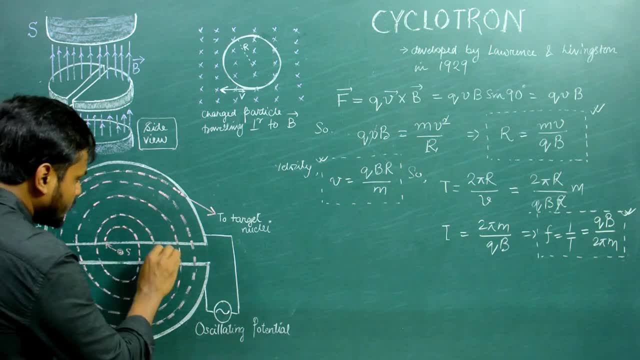 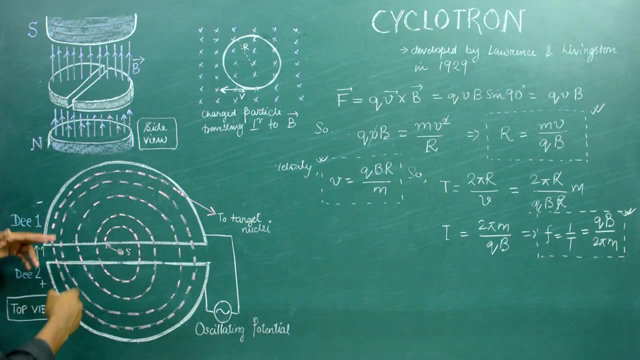 be in this particular direction, All right. So at every point in space there is going to be an electric field in this upward sort of a direction. So every time the polarity gets reversed, the electric field in this region also gets reversed in its direction. 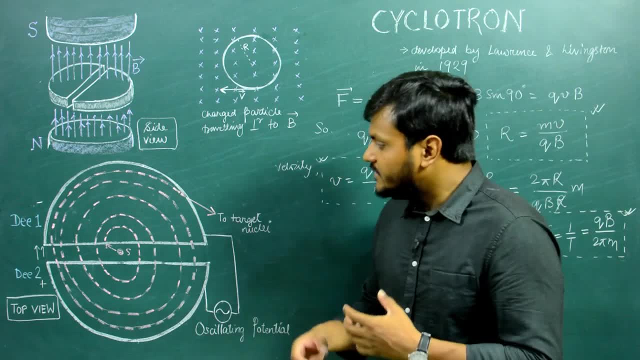 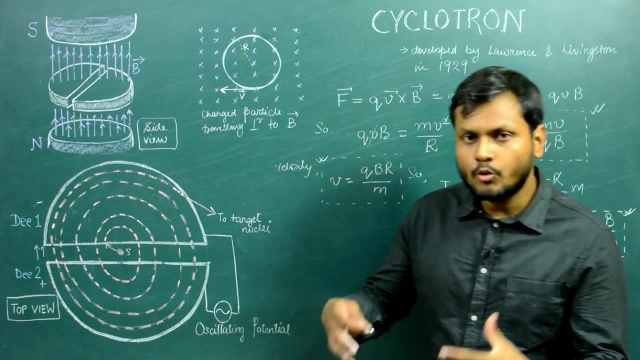 Now what happens because of this? Let's suppose that there is some sort of an ion source at the center here that emits some kind of an ion. let's suppose a proton particle. All right, Now, once the proton particle is emitted, the proton particle experiences the electric field in the upward 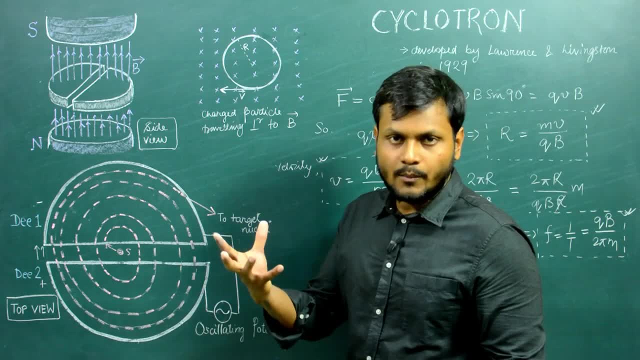 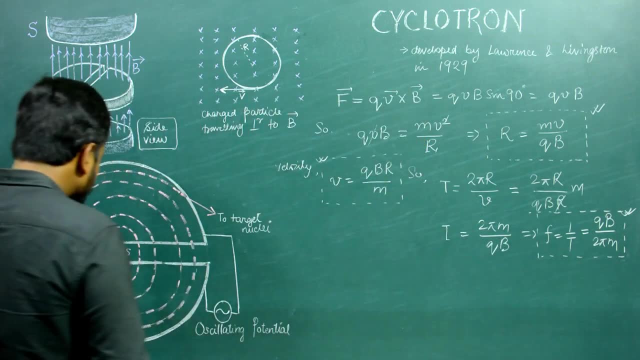 direction? Yes, and then the electron particle is emitted in the upward direction. So let's suppose that thisalanium was also released from thisfalon, the NING. So as a proton particle enters the electron position, the crescent Star entrance time as it does, 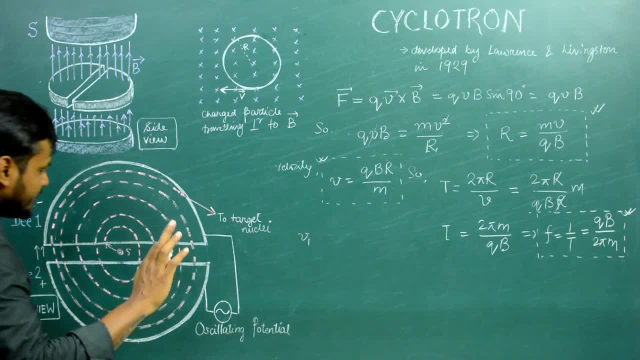 access the electron from that point of time is now equal to 2.5 Stop الف, And it's getting accelerated in the upward direction. So as it gets accelerated, it basically enters… Let's suppose, D1.. So, as the charged particle enters D1 after experiencing, some sort of an acceleration. let's suppose it enters D1 with a velocity of v1.. Now, what is interesting is that the moment the charged particle enters D1, now because inside this half of a cylinderud Democrats, Four Cylinders are both stable in save or observe, as itadora, The potential is constant-Yes, and 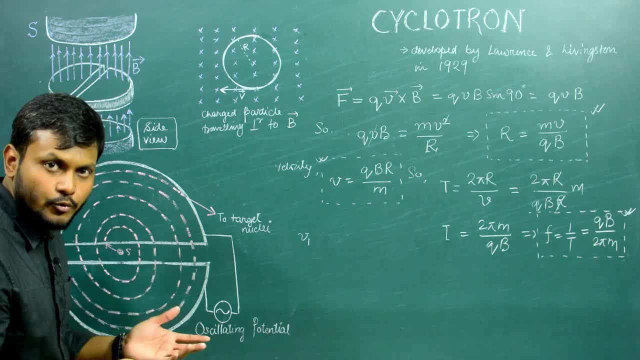 because of this function, because of this function of the electron and the weirdly factors that are facilitate every electron can express only real power. 에�chezp del-dp. Because the potential is constant, the electric field is zero. The electric field is only non-zero. 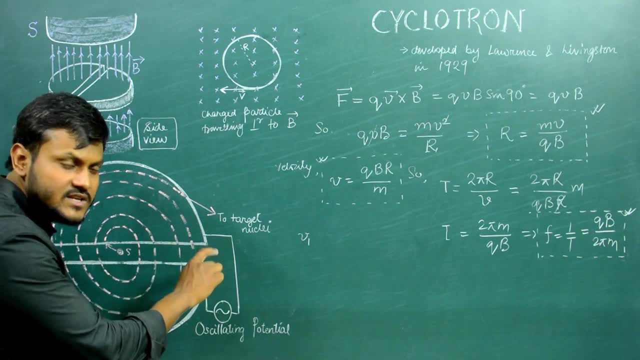 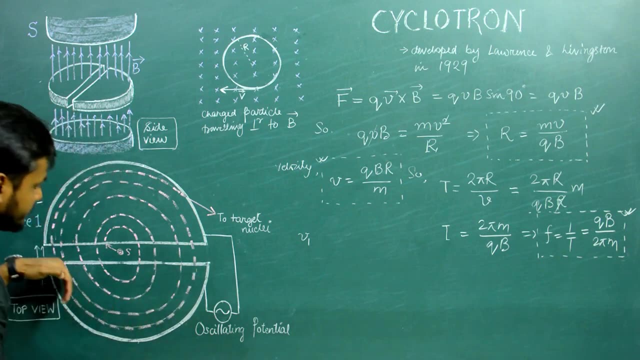 in this space where there is a potential difference. But within the cylinder itself, where the potential is constant, the electric field is zero. And the same here also Within the cylinder itself, where the potential is constant, the electric field is zero. 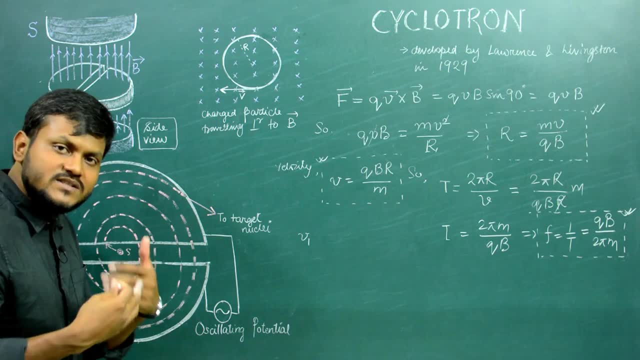 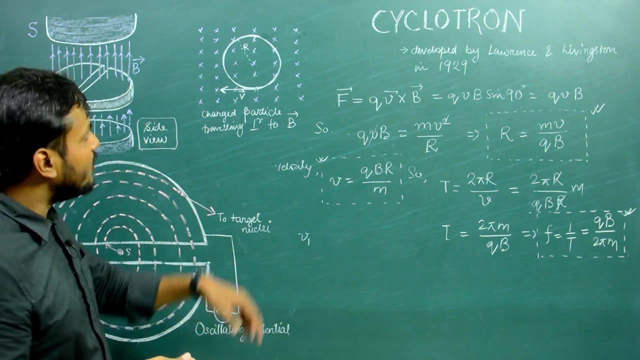 So as the charged particle enters D1,, in that case, because the electric field is zero, it does not get accelerated anymore, It retains a constant velocity. Now, what happens because of this constant velocity? as we already discussed, There is a magnetic field line. 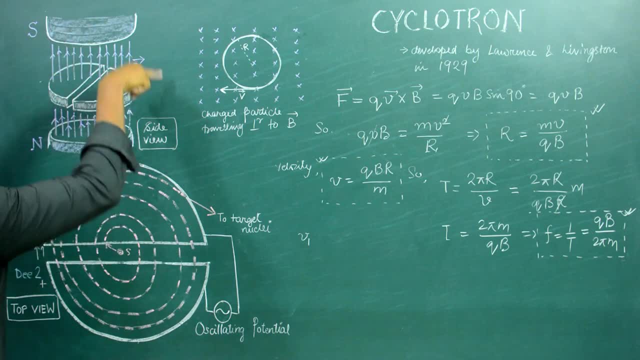 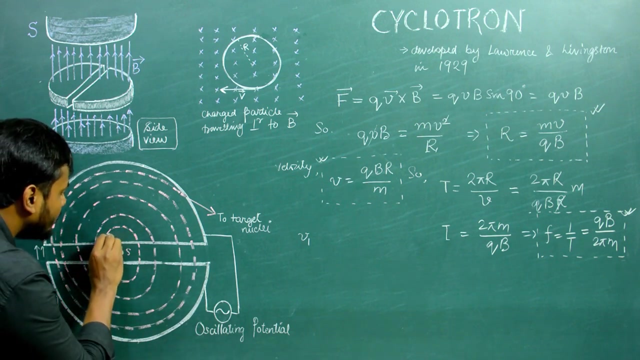 which is going from north to south pole in this view. But in this view the magnetic field lines are basically coming out of this board. So there are magnetic field lines coming out perpendicular to the plane of this board. So because of this, this kind of a charged particle as it enters D1,. 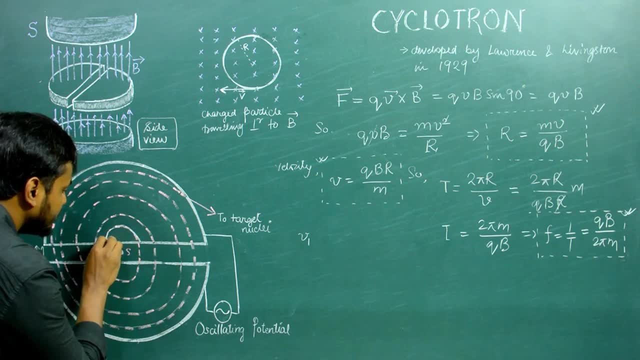 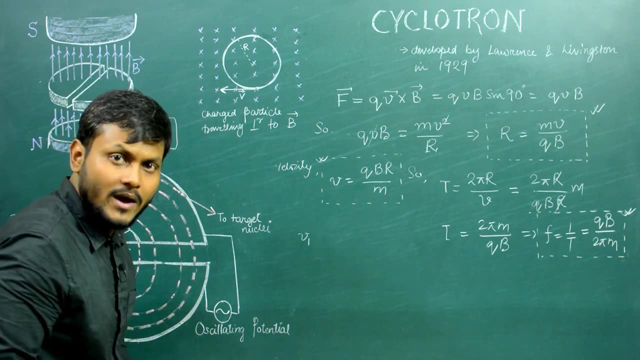 will execute a semicircle, you can say So. it will execute a trajectory of a circle, And then again, Again, it will come out of D1.. Now, the moment it is about to come out of D1, let's suppose 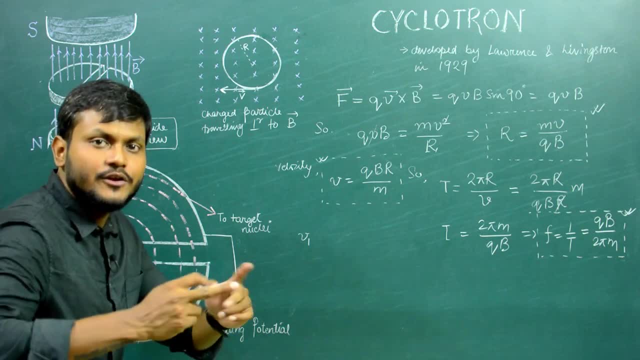 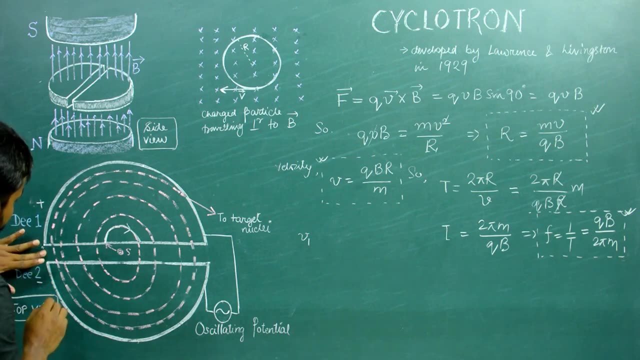 the polarity of this oscillating potential reverses. So if the polarity of the oscillating potential reverses, this becomes positive and this becomes negative. Now, suddenly, the electric field is also in this particular direction. Yes, So electric field is now facing downwards. So 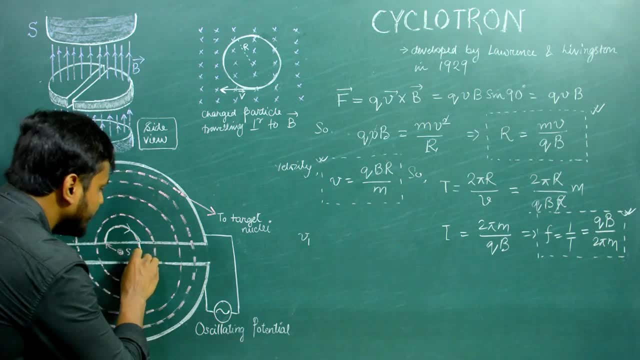 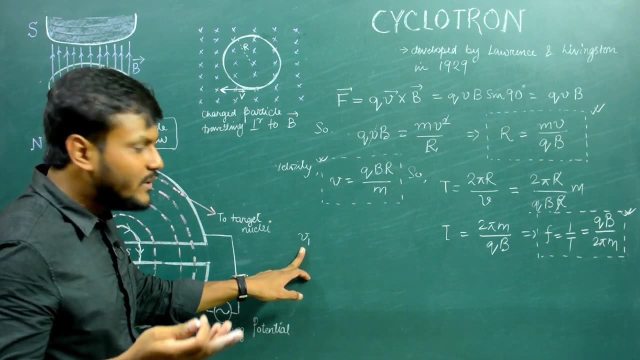 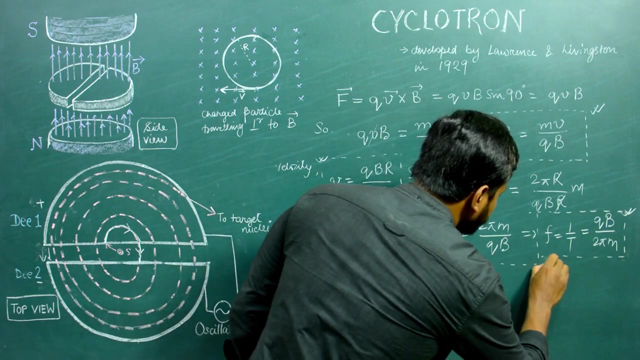 now this charged particle will get accelerated in this particular direction. Yes, Now, because it will experience acceleration. its velocity is going to increase and we can calculate what is the change in the velocity. So change in the velocity can be just looked about from the change. 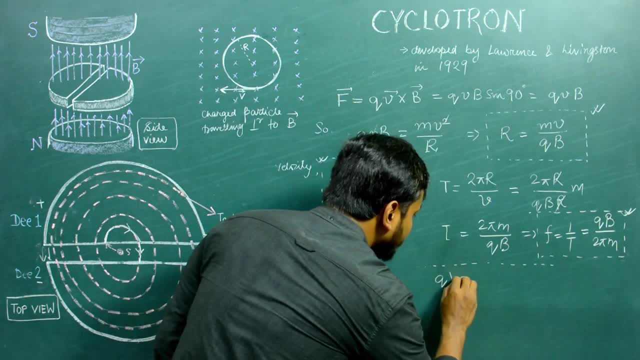 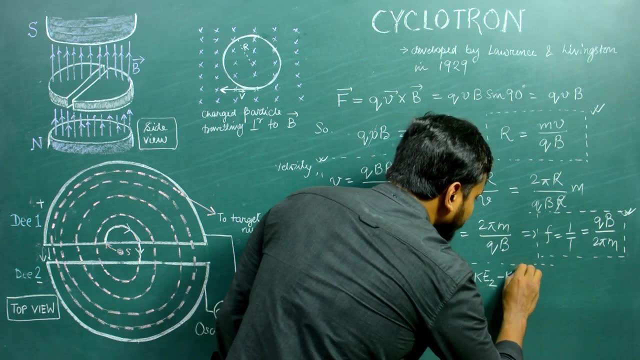 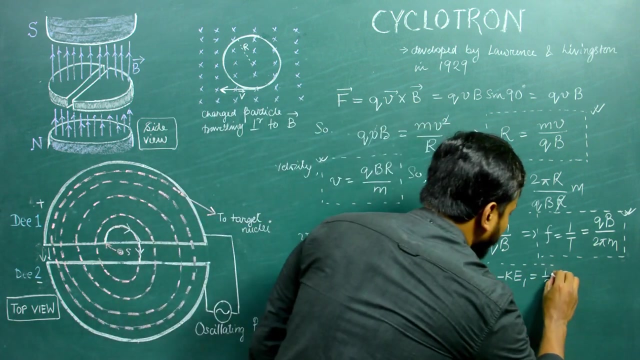 in the kinetic energy. So basically, the potential can result in the change in kinetic energy which is equal to QV. This is nothing but the final kinetic energy minus the initial kinetic energy. Yes, So if let's suppose the particle had initial velocity V1, it will have a new velocity V2, where the change is half. 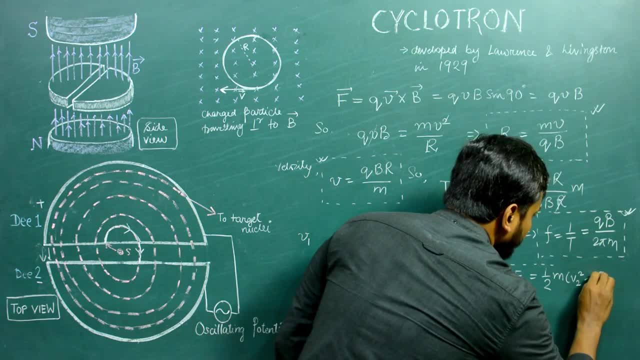 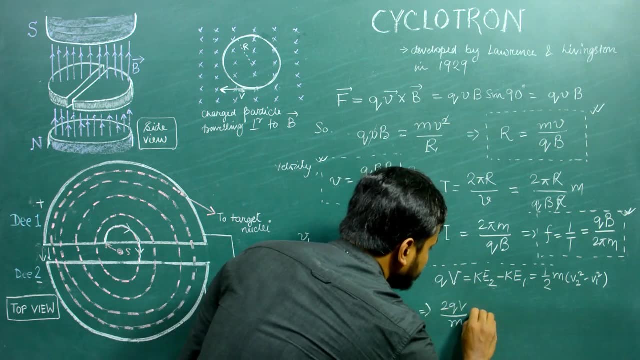 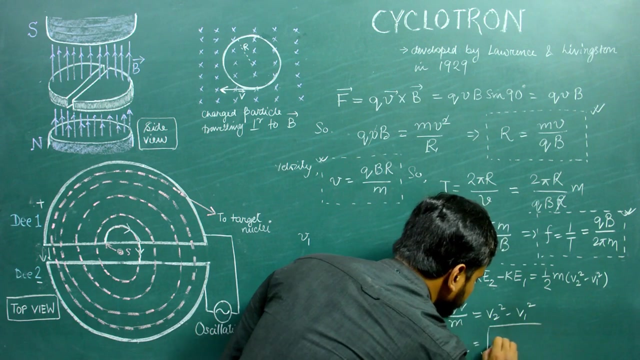 m V2 square minus half m V1 square. So this can be written as: 2QV upon m is equal to V2 square minus V1 square, or V2 is nothing but root over V1 square plus 2QV upon m. So basically if 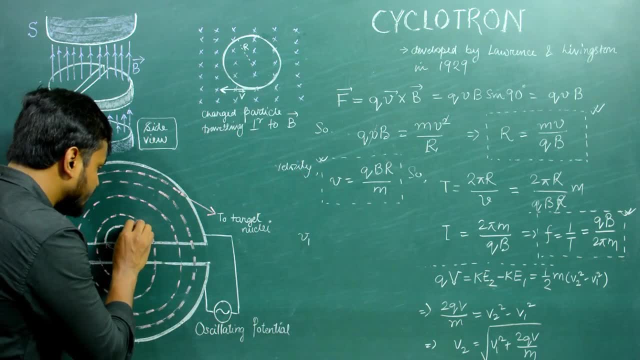 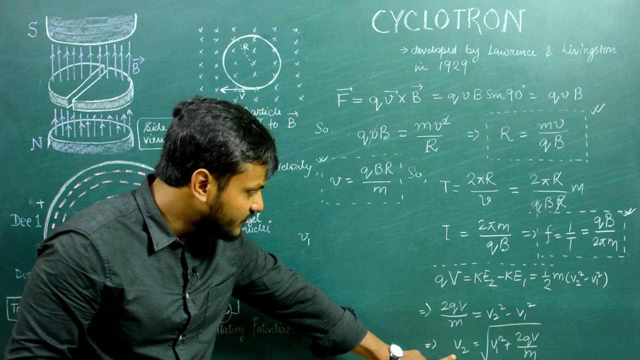 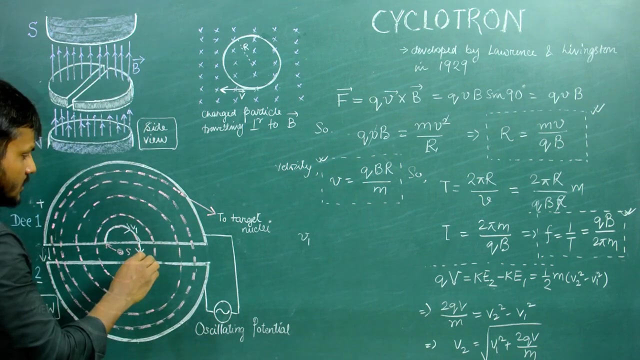 the charge particle had V1 velocity here. then the moment it experiences a potential difference of V, its velocity increases to V2, where V2 is equal to root over V1 square plus 2QV upon m. So basically it increases by a certain amount. Now in D, number 1, because of velocity V1,. 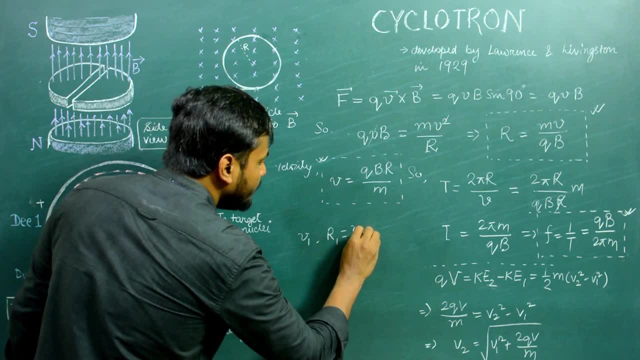 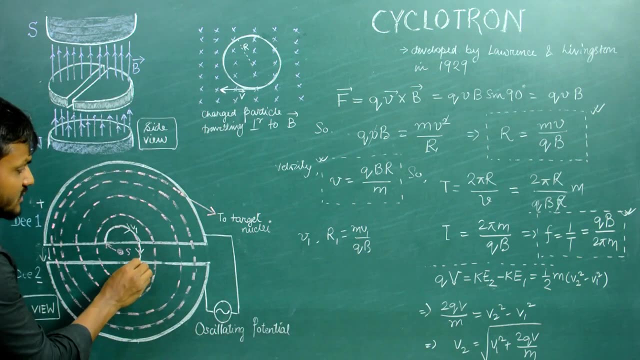 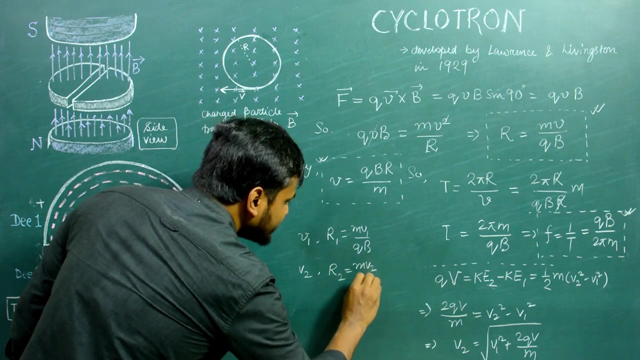 the charged particle had a radius R1 of m, V1 upon QB. As it enters D2, its velocity increases. And now, because velocity increases to V2, now the radius corresponding to V2 is also greater. yes, So the radius corresponding to V2 is greater than the radius corresponding to V1. 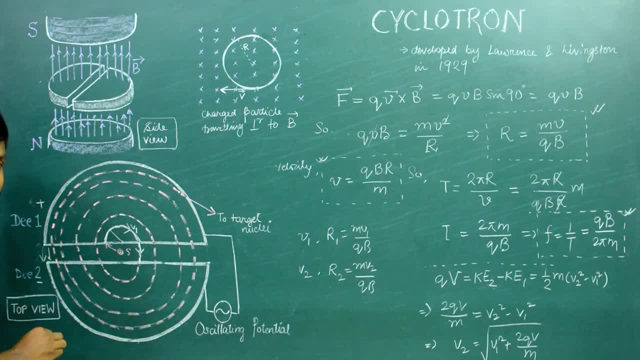 So the radius corresponding to V1 was this radius, yes, But now because of the acceleration, the velocity has increased and the radius corresponding to V2 is of this, basically radius. So now it executes a circular trajectory, but that has a radius greater than the earlier circular trajectory. Now, 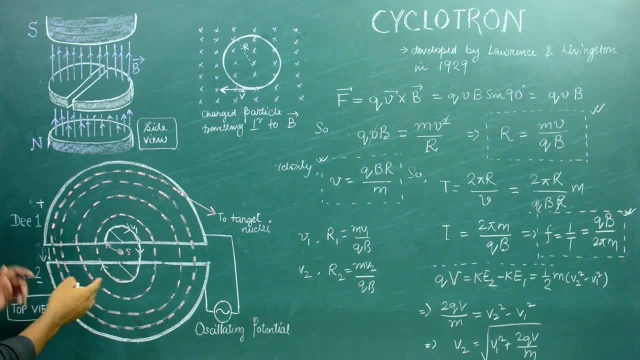 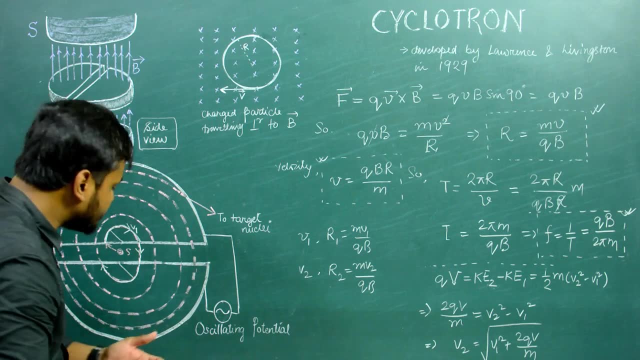 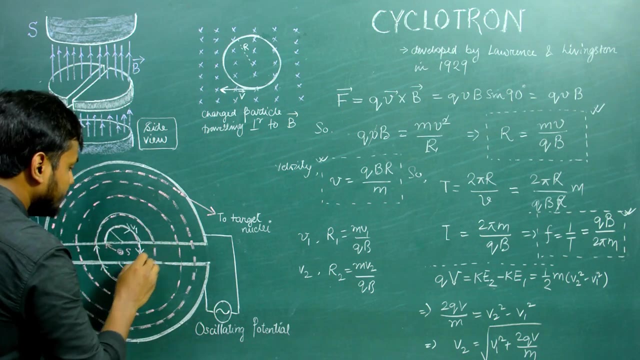 again before it is about to exit d2. again, let's suppose the polarity gets a reverse, so this becomes negative, this becomes positive and the electric field also gets a reverse in direction. so again it accelerates, and then again it has a larger sort of a radius of a circle. then again, 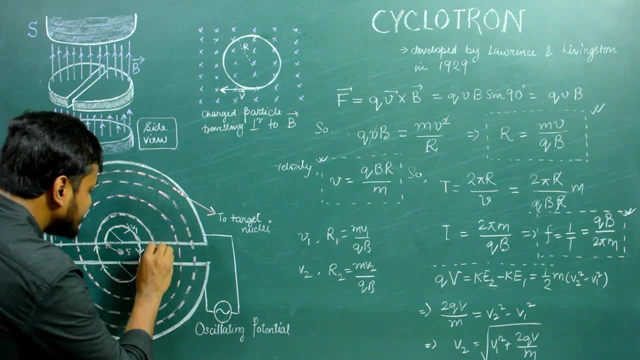 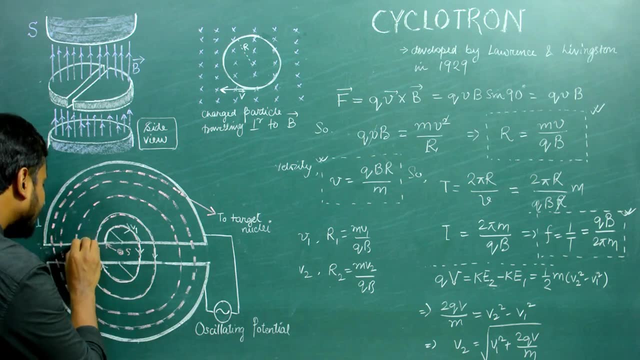 the polarity reverses right, and again it gets accelerated, and again it executes another larger sort of a semicircle. then again the polarity gets reverses, reverse, again it accelerates, again it experiences a larger semicircle. so this process keeps on happening, over and over again. 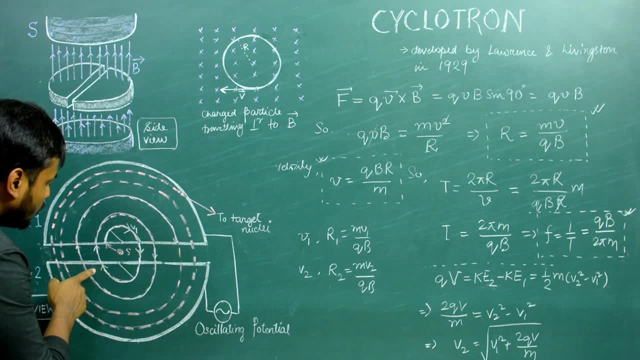 so that at every time the particle is about to exit any one of the d, the polarity is reversed so that the particle only experiences an electric field pointing in the direction of its motion, so that the particle gets accelerated and its velocity gets increased consecutively. so if the 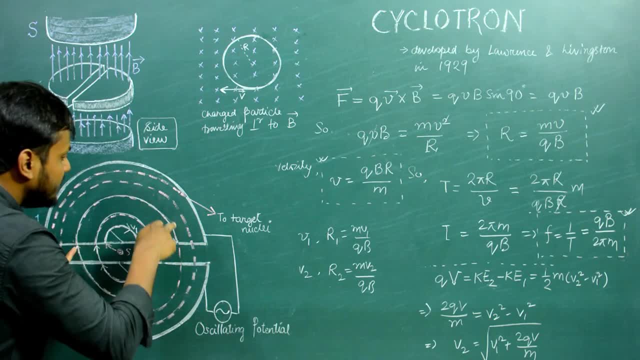 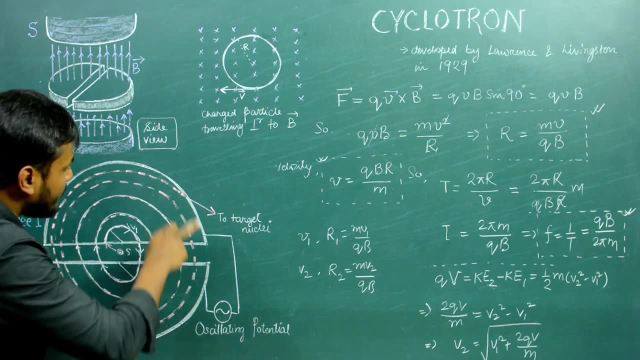 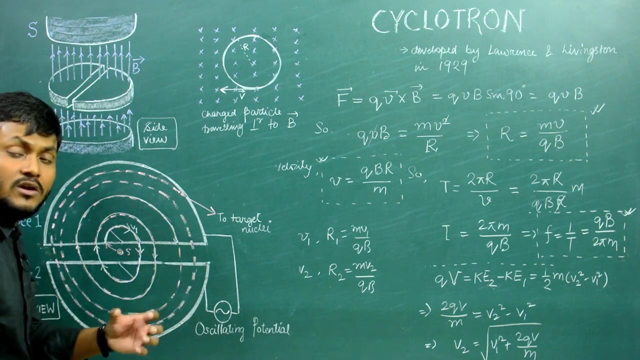 velocity gets increased. now now the radius executed by its trajectory will also be greater. so the particle keeps on going with increasing semicircular radius. so basically it keeps on going in this kind of a spiral sort of a trajectory. with every step it goes on, its velocity keeps. 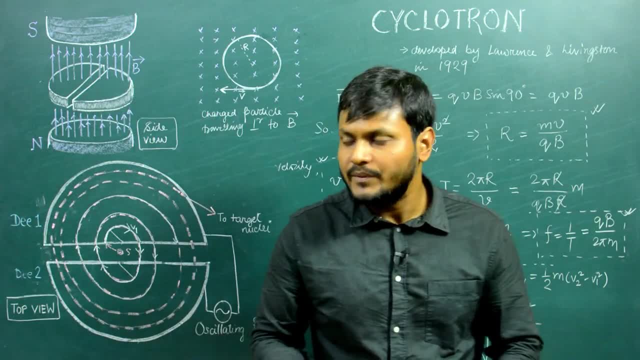 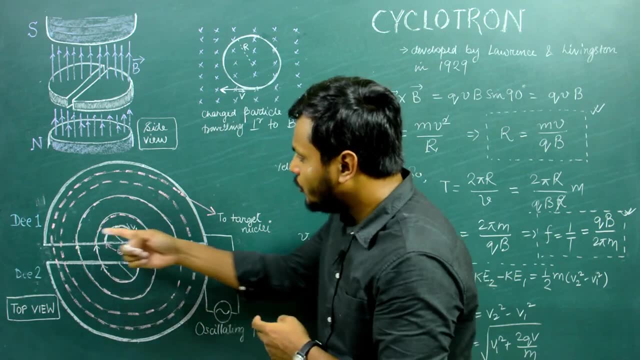 on increasing. so this is how the whole process keeps on happening inside the d. the particle executes a semicircular motion. as it is about to exit the d, the polarity gets reversed, so the electric field is now pointing in the direction of the charged particle. so the charged particle 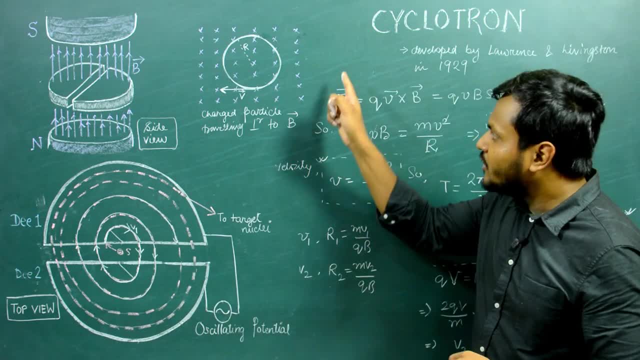 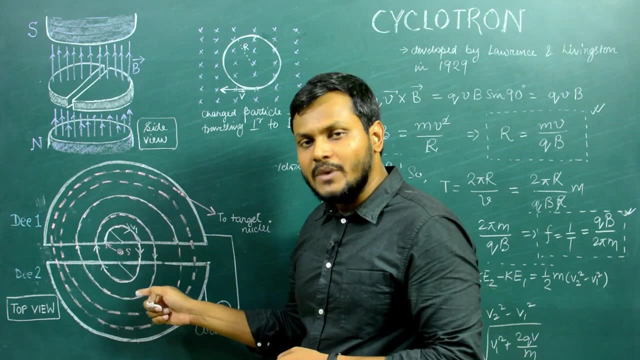 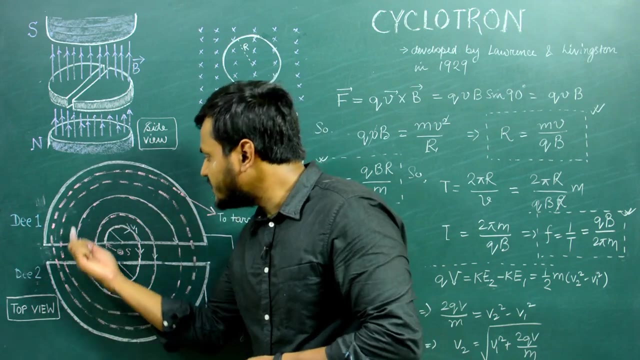 velocity increases and the corresponding radii of that circular trajectory increases. so now again it executes another circular motion. there is no acceleration within the d's because the potential is constant. here and again, as it is about to exit, the polarity reverses, it experiences an acceleration. so every time the charged particle enters a region between these two d's, it gets. 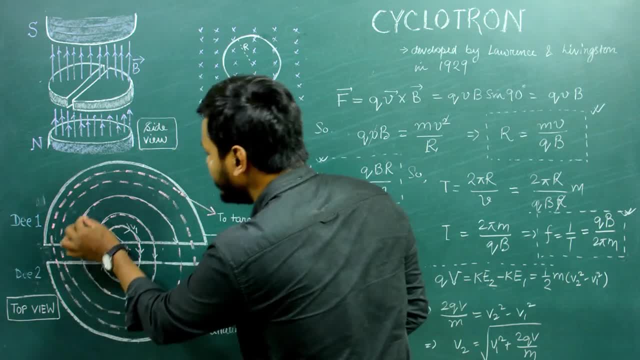 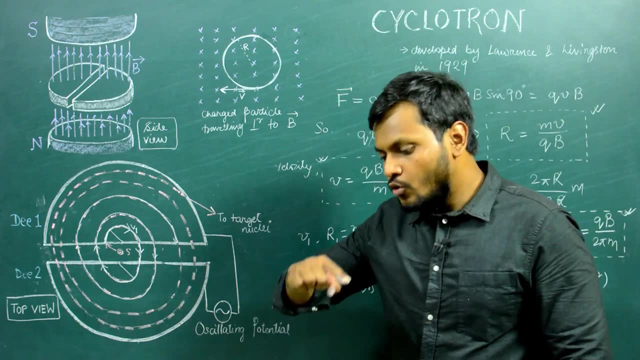 accelerated, and then again it gets accelerated, again it gets accelerated, and again it gets accelerated, over and over and over again. so the charged particle as it goes in a circular motion with increasing radii. so basically it's going in a spiral motion, it keeps on increasing its 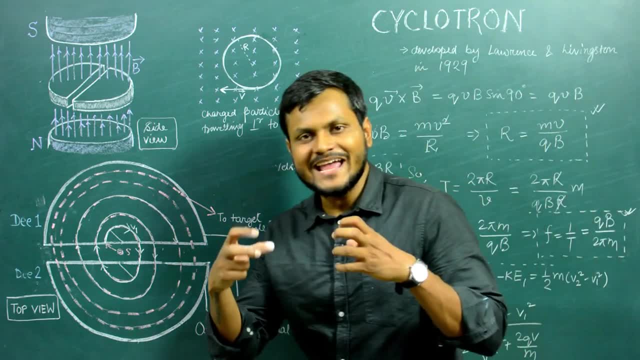 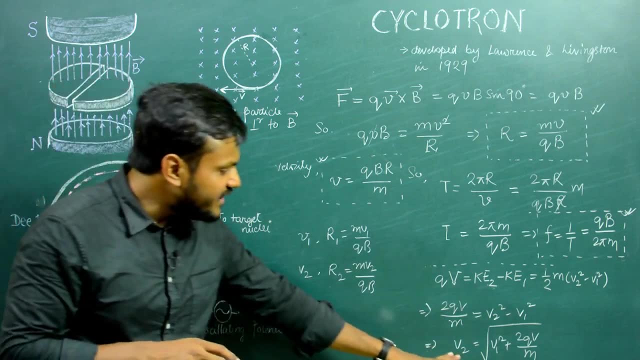 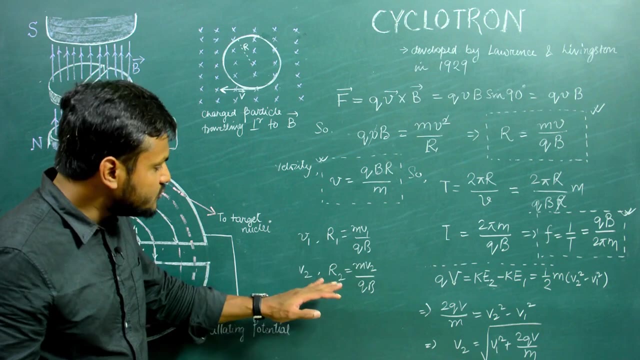 velocity, over and, over and over again. this is how the cyclotron increases the velocity of a charged particle in a very compact sort of a space, thereby reaching very, very high values after many number of accelerations. here i have calculated r1 and r2, but similarly you can also. 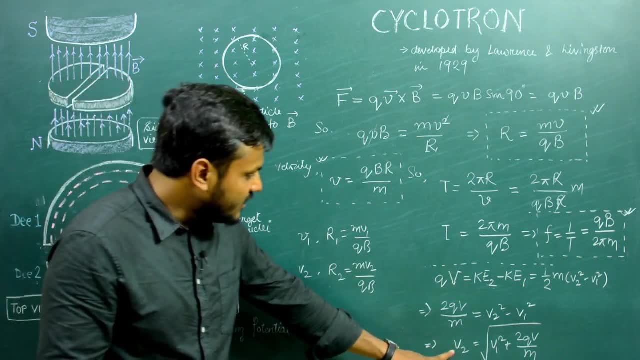 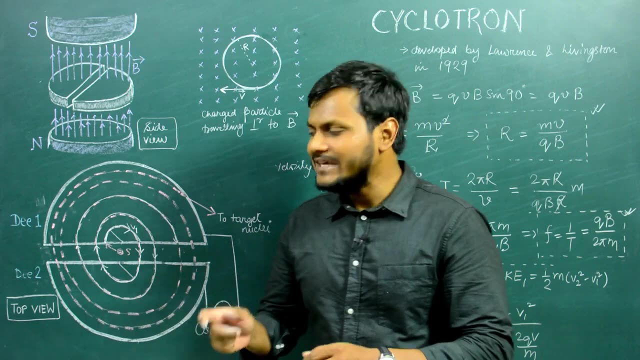 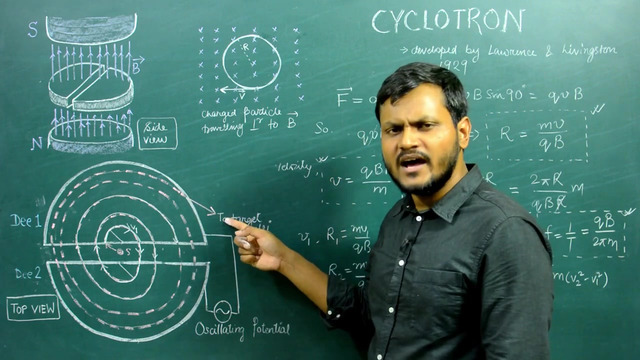 calculate r3, r4, r5, r6, and here you can calculate v3, v4, v5, v6, where at every step the radius and the velocity keeps on increasing, thereby reaching a certain value that, when it is about to exit, it has extremely high velocity. that means it has extremely high kinetic energy. so that now this 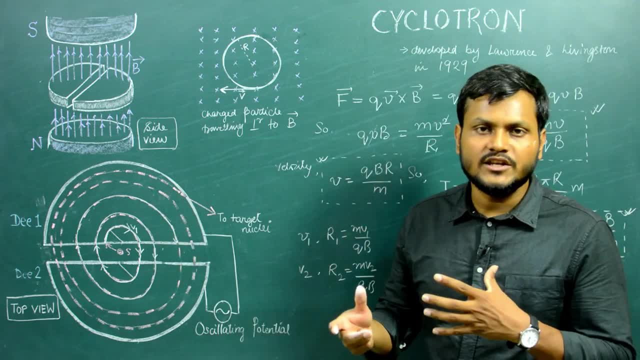 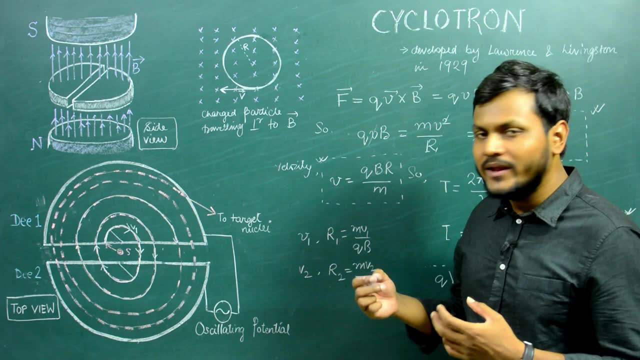 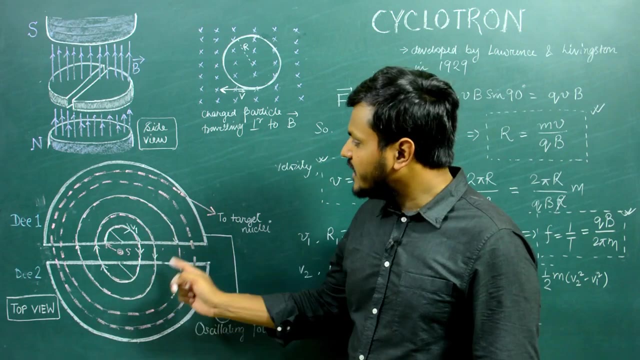 kind of a charged particle can be targeted to some sort of a target nucleus to perform some kind of a nuclear experiment. so this is the general working mechanism of a cyclotron, that when a charged particle is placed in the presence of a magnetic field it tries to move in a circle. in this case it is placed also in the presence of two d's which 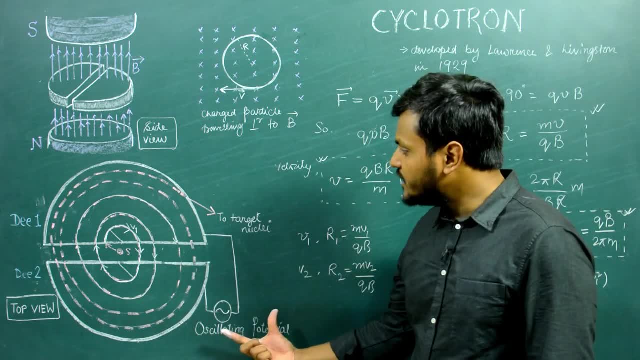 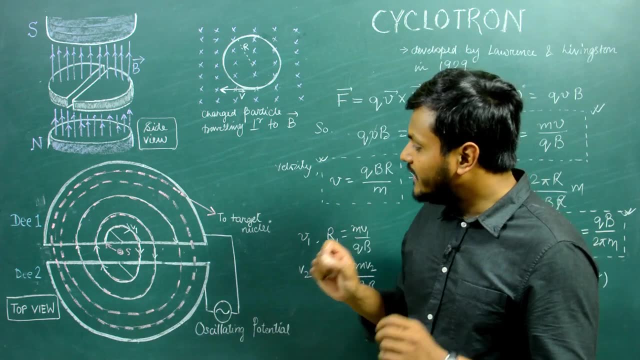 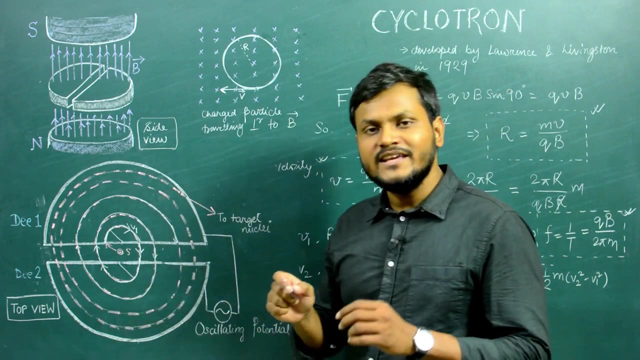 are connected to opposite polarities of an oscillating potential, so that every time it comes in between these two spaces it gets accelerated. now one thing has to be clear: that every time the charged particle is about to exit, the polarity gets a reverse, so that the electric field is always pointing in the direction of the magnetic field and the electric 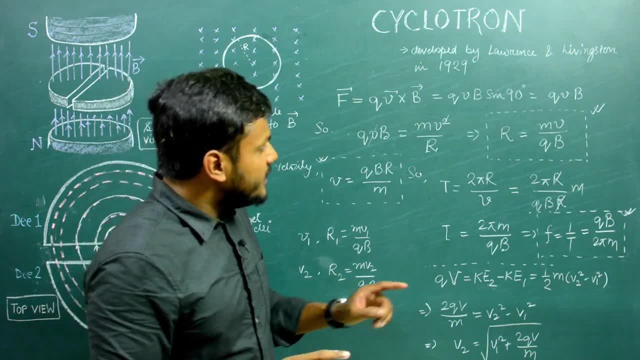 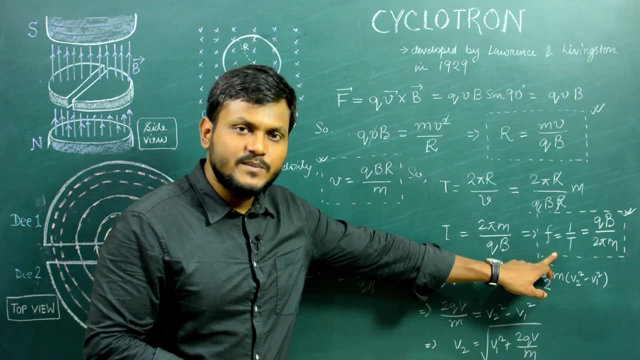 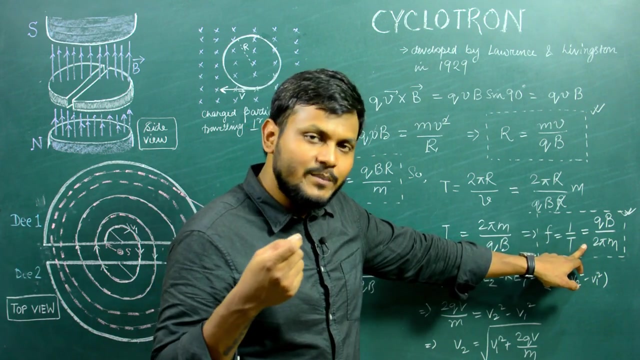 field is pointing in the direction of the charged particle. this can only happen if the frequency of oscillation is basically equal to f here. so f is basically the frequency of revolution of the charged particle. as you can see, this is independent of the velocity. this is also independent of the 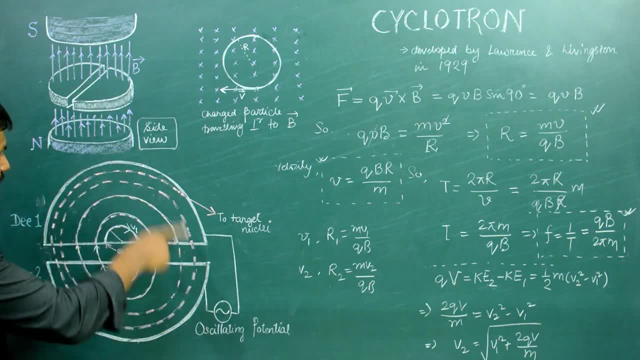 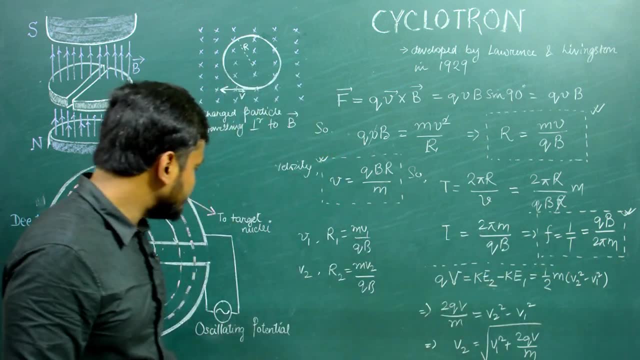 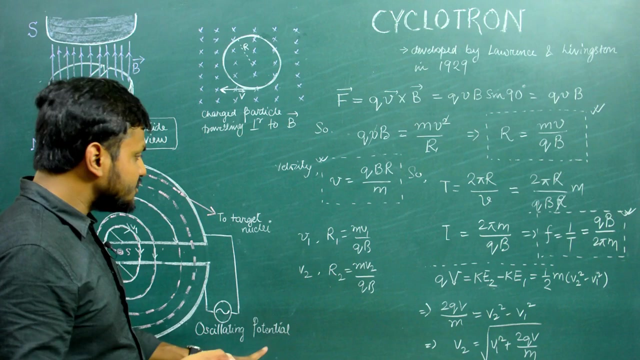 radius. that means at every single point, the frequency of revolution of the charged particle is this: it is independent of velocity and independent of radius. so if we can match the same frequency- oscillating potential, So this is basically known as resonance frequency. So if we can match the 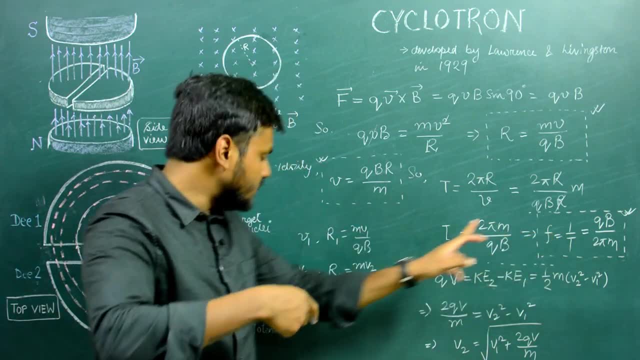 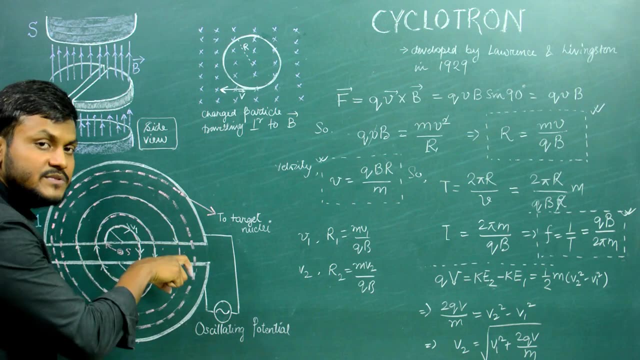 frequency with which the charged particle is making revolutions with the oscillating potential. then we can make sure that every time the charged particle is about to enter this empty space, then it will always experience a positive electric field in the direction of its motion. So this is 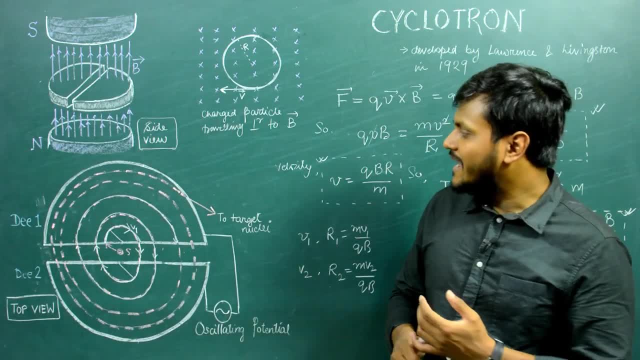 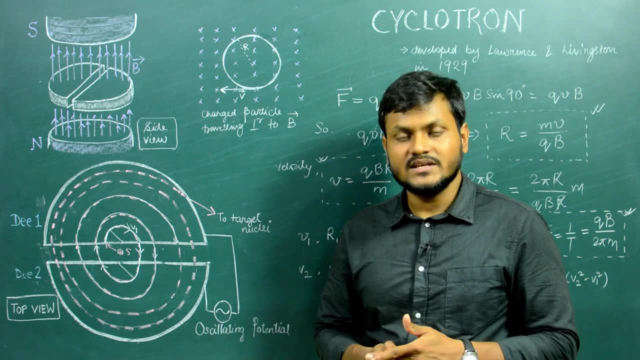 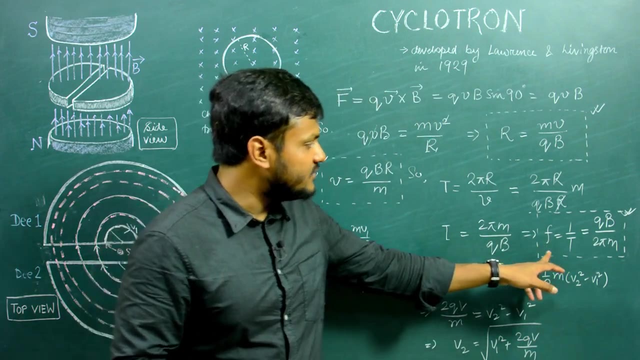 in general how a cyclotron works. However, it has a particular disadvantage that an extremely high velocities it reaches relativistic speeds. then the frequency changes. So for example here I have: the frequency which is given by f is equal to q capital b upon 2 pi m right. So the frequency here. 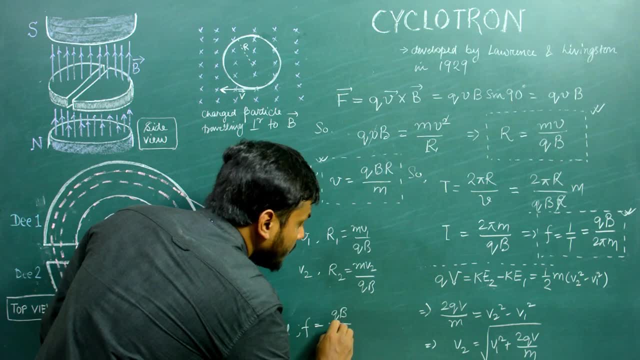 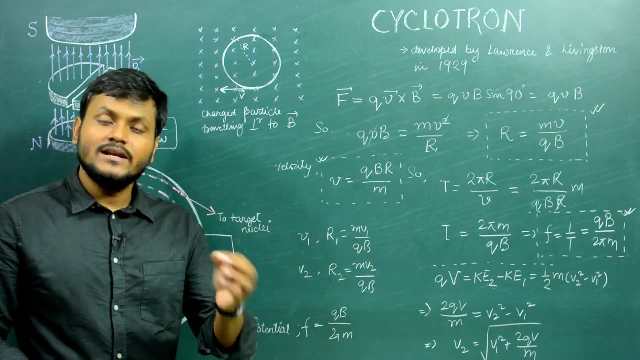 is basically q capital b upon 2 pi m. Now, as you know that at very, very high velocities, near about the velocities of the speed of light, there is a relativistic increase in the mass of the charged particle. So if there is a relativistic increase, 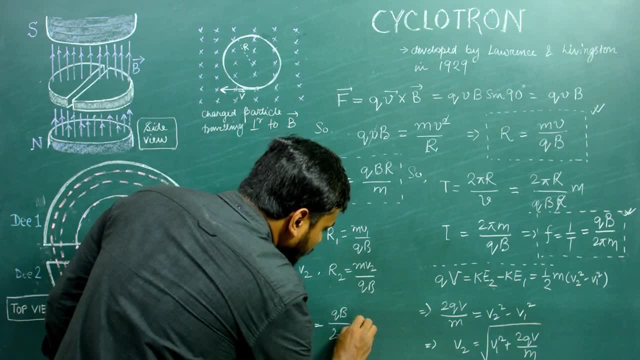 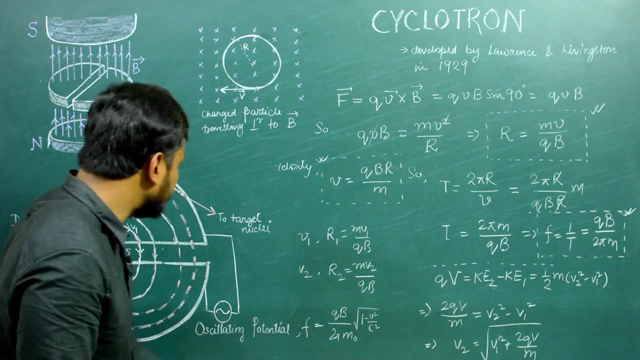 then I can write the increase in relativistic mass to be m naught root over 1 minus v square by c square. Now, because of this, what happens is that at very, very high velocities the charged particle starts slowing down. So as the charged particle starts slowing down, the resonance 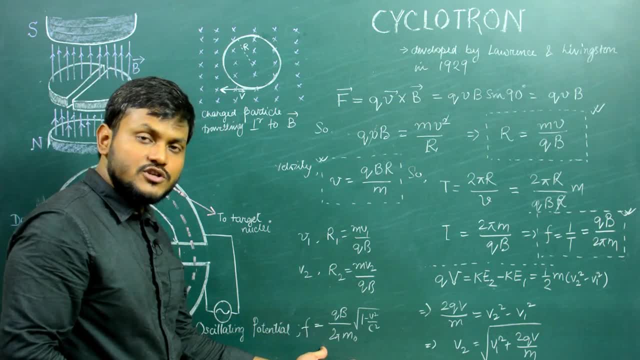 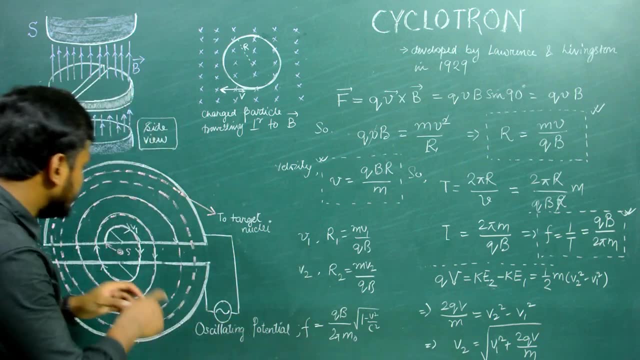 frequency of the frequency of revolution of the charged particle does not match the frequency of the oscillating potential. So the charged particle starts lagging behind this kind of a potential and it does not get as much of a result as the charged particle does. So if we can write the 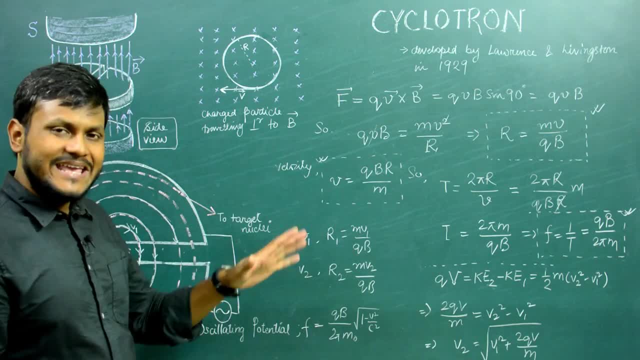 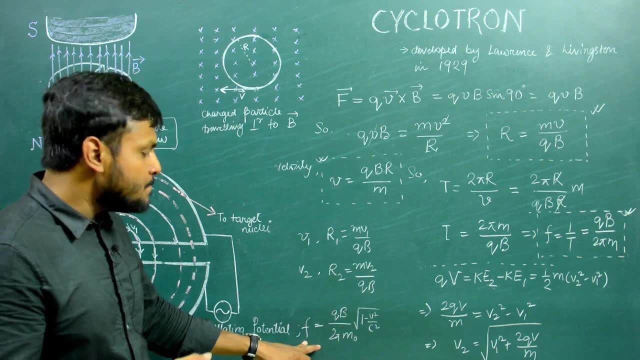 uencia of acceleration, in other words the fact that there is an oscillation. there is even a small shift of Mozambique with the partager ‑‑ right why i Photo might be aaks on the mic caused by the stronger vibrational power of the c? clock. then C are found to be. 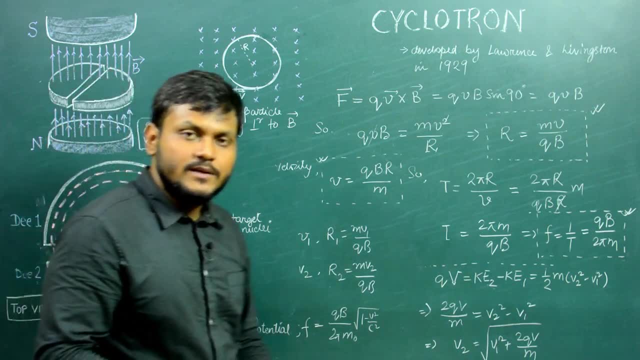 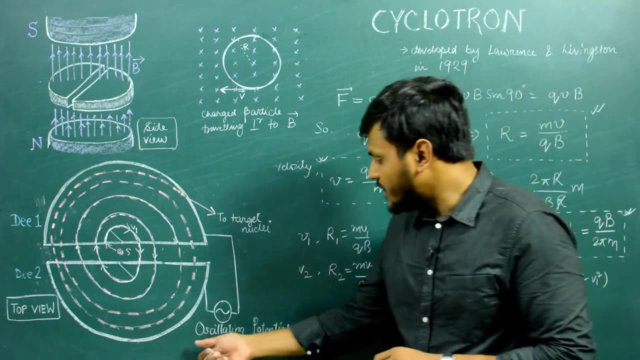 Ч Are found to be at scattered at randomly in time. so therefore cyclotrons cannot work in relativistic speeds, because in relativistic speeds we end up getting a frequency which changes as the particle reaches very high values and that frequency does not match the frequency. 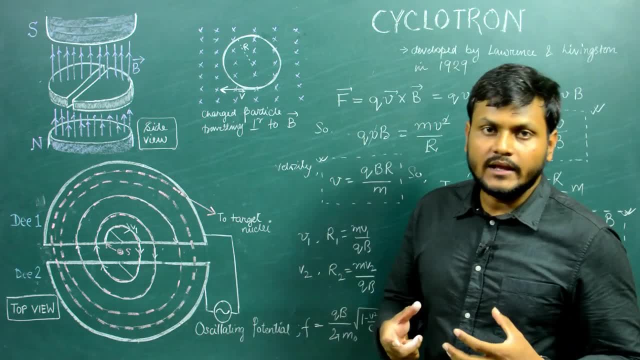 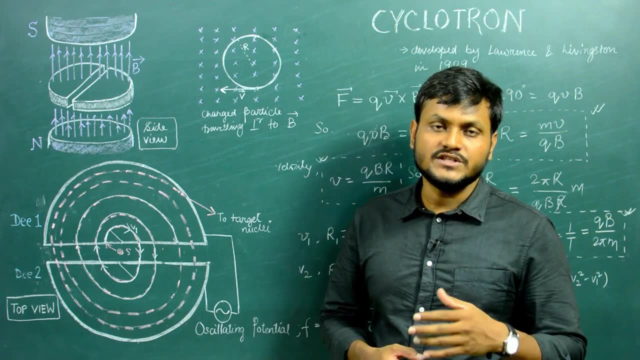 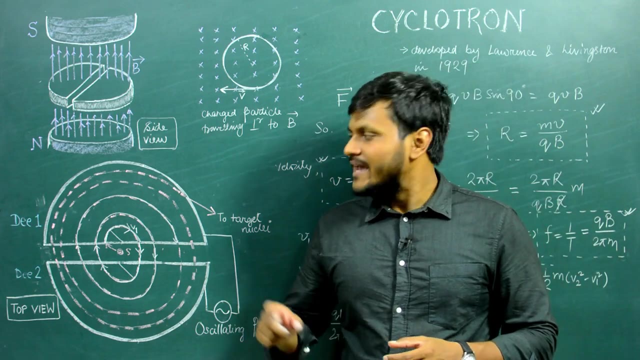 of the oscillating potential. And then 축 is a very common particle accelerator that can reach very, very high values, hundreds and hundreds of mega electron volts of energies for charged particles like protons. The only disadvantage is that it cannot work in relativistic speeds. When cyclotrons are modified to work in relativistic